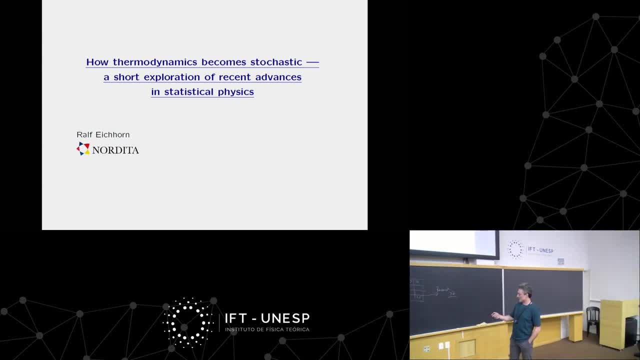 Okay, As I said, the title of my talk is How Thermodynamics Becomes Stochastic- a Short Exploration of Recent Advances in Statistical Physics. And, of course, Such an exploration can only be subjective, So I'm going to present some recent advances from the perspective I'm interested in. 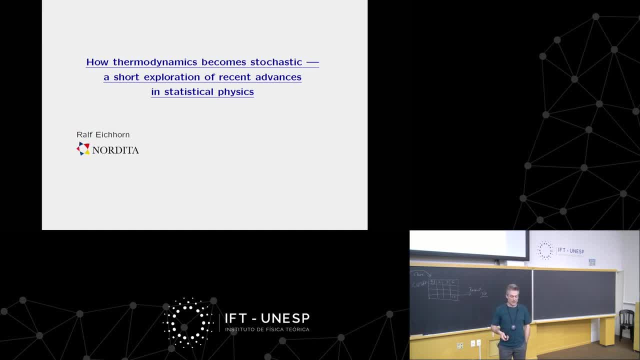 So it will be a selection. I cannot, of course, cover everything that happened during the last, say, 10,, 20 years, But I will try to give you a flavor of what I think is a very interesting development in statistical physics. 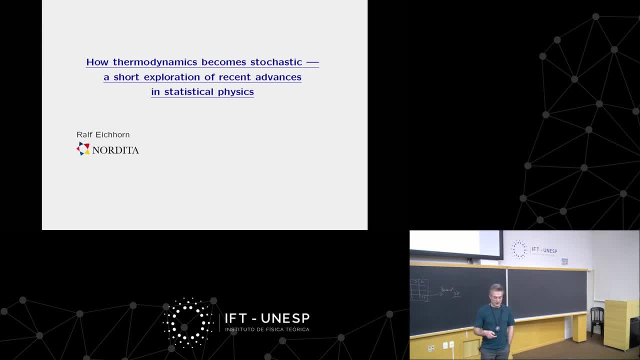 And for those who are participants In the school. the talk is also, in parts at least, a summary of my lectures, But it will go beyond my lectures too, So I would like to start with the second law of thermodynamics. 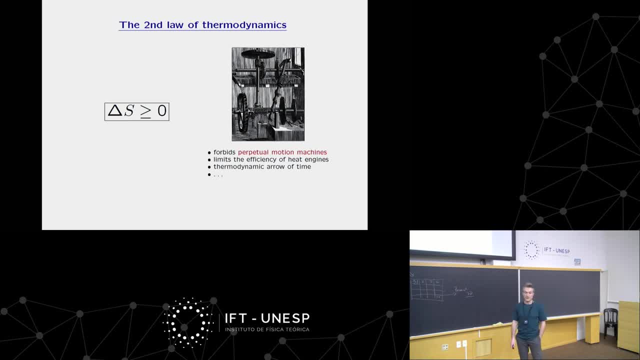 This is a formulation which we most often use to write it down- That the change in entropy has to be positive Or not negative. let's say- And this is a very important law, We know that, We know that, We know that. 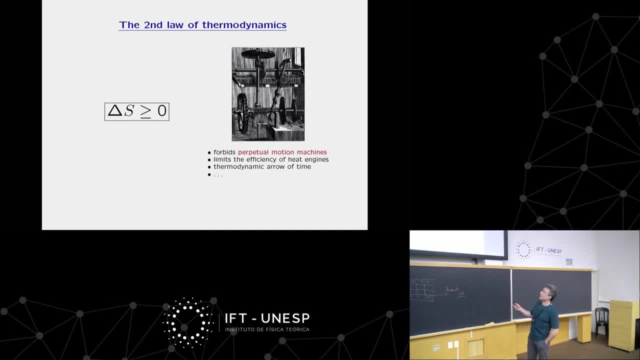 It forbids, for instance, perpetual motion machines here. I mean, if you Google you'll still find people who try to build these kind of machines And there's an old picture of someone who tried. Then it limits the efficiency of heat engines. 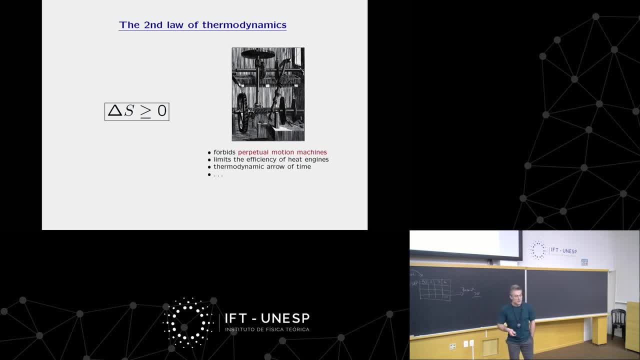 Probably the most important practical implication. It's related to the thermodynamic error of time and so forth and so on. So it's a very important law. So let's recall what this means We have. We have a system in equilibrium, a thermodynamic system in equilibrium which has a certain entropy. 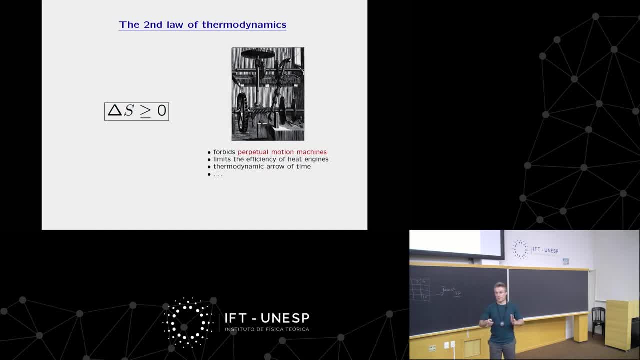 And then we remove a constraint, something that limits the ability of the systems, And then we let We relax it to a new equilibrium state And if you compare these two states, the entropy change is not negative, And a typical example of that is a gas. 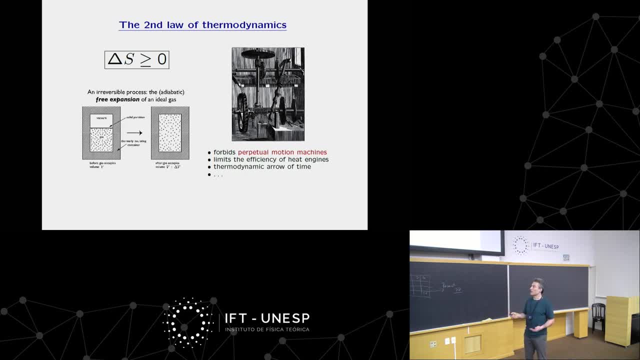 In some kind of container where there is a wall in the very beginning. This is the constraint which limits the, Which constrains the gas to a part of the container. When we remove that constraint it can expand and will have a different entropy. 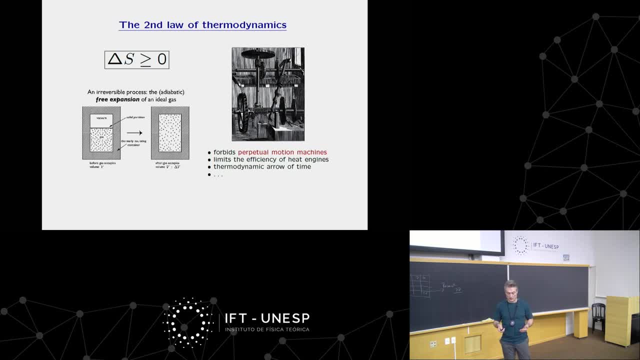 And the change in entropy is not negative. This is the second law, But if you think about it, of course this expansion process here is not always the same, Because the gas molecules they're moving Not in exactly the same way. 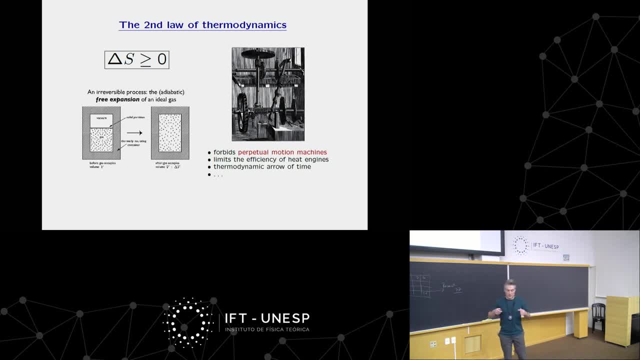 So if we repeat the experiment, in principle we have to take into account that there are fluctuations in this whole process. But we also learn that these fluctuations for macroscopic systems are unmeasurably small. So in principle we should write that the average entropy averaged over many repetitions of this experiment is non-negative. 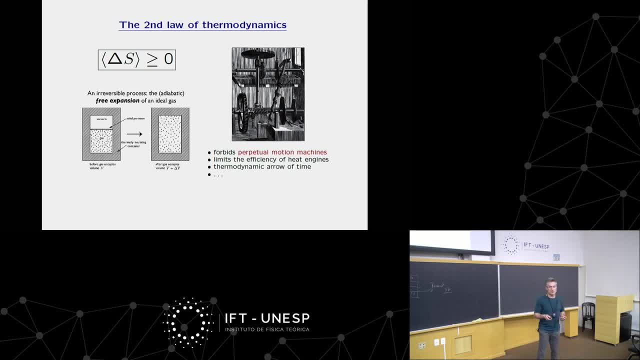 But for a macroscopic system it doesn't actually play a role, Because the fluctuations scale down with one over square root of the number of particles involved, And this is typically 10 to 23 or something like that. But what if we look at systems which are made of not so many particles, of much less particles, maybe just one particle. 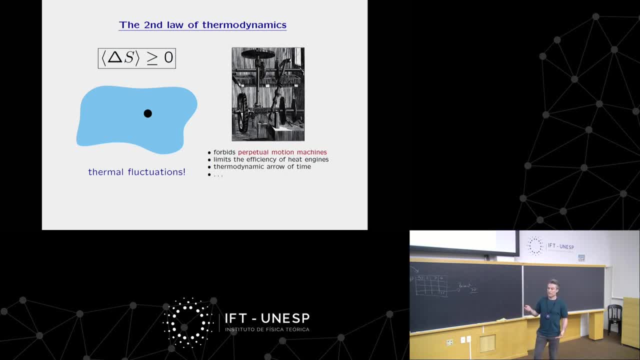 This is what we're discussing at the school in part. So my Favorite example here: Just one particle, this thing suspended in an aqua solution, A colloidal particle, Just this one particle, And this we know now, is subject to thermal fluctuations. 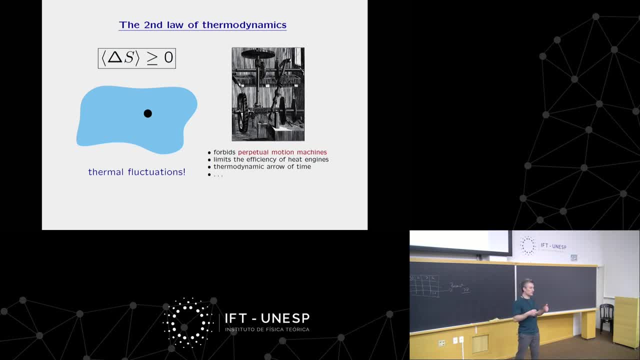 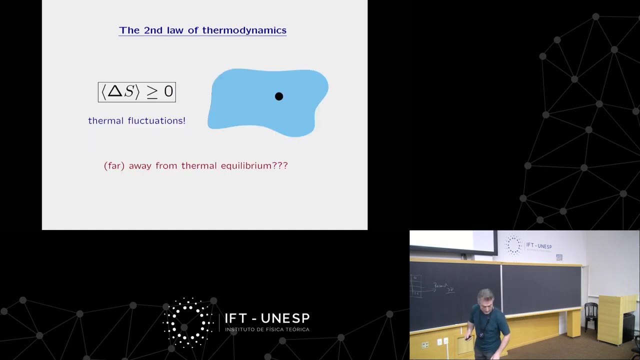 This is of the size of a micrometer. So small systems, one particle, small systems subject to thermal fluctuations, which actually play a dominant role in these systems. So what happens then to this average entropy production? Even worse, if there are some driving forces which drive this system, this particle. now, the particle is our system, it's in contact with a bath, it can equilibrate with a bath, but there can also be driving forces, gradients and temperature gradients and chemical potentials, external forces, electric fields and so on, which drive the system away from equilibrium. 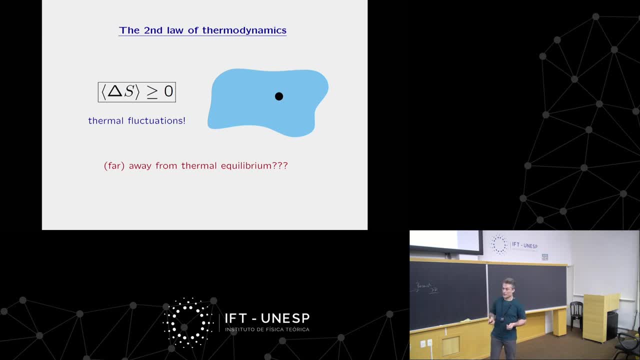 Which don't allow the particle to equilibrate with a bath, What happens? But then can we still speak of entropy? We know entropy is an equilibrium concept, right? So can we even define changes in entropy for such a system? And this is what I would like to discuss with you during the lecture: that this, if you do it properly, is indeed possible. 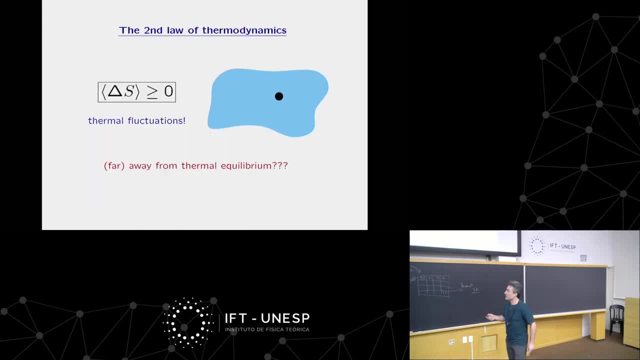 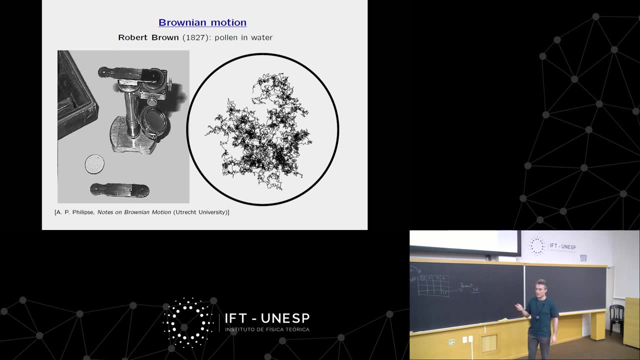 And as said, this particle here by the thermal fluctuations does this Brownian motion here. And just a very, Just, a very few words on Brownian motion. You know already it has been systematically studied by this botanist, Robert Brown. 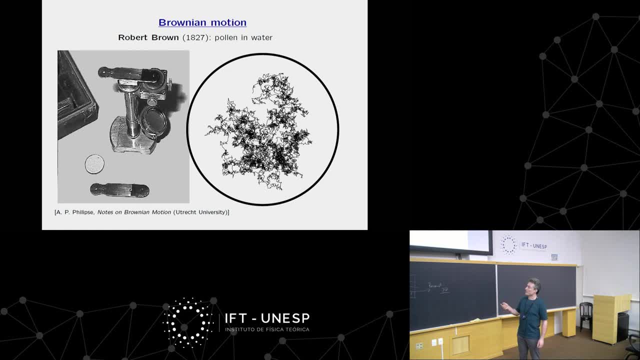 That's the reason it's named after him, And he used a microscope like that and observed for a Brownian particle something like that. So this is the wiggling motion I'm talking about. This is the effect of the thermal fluctuations. This is how a trajectory of this single colloidal particle under microscope would look like. 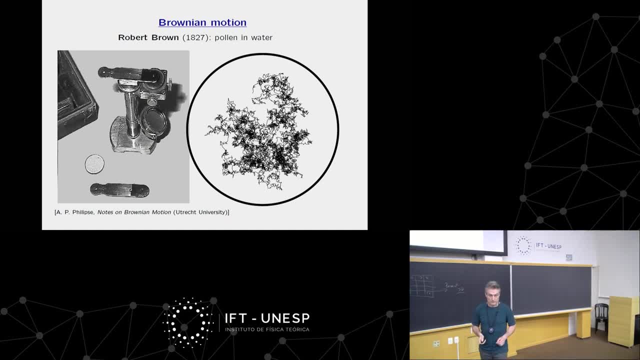 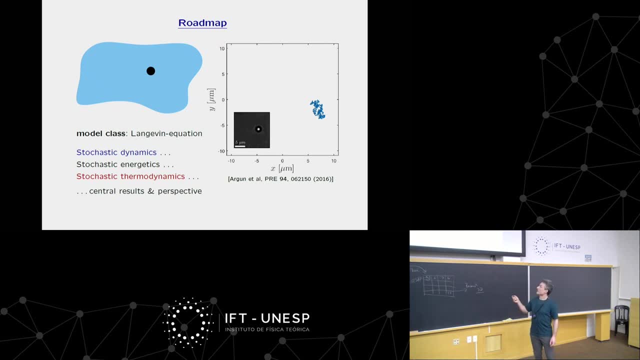 Here. this is actually not a real observation. This is created by a simulation, But I have also real measurements on that slide here. This is a real experiment. This is the colloidal particle. This is in the group of Giovanni Volpe in Gothenburg. 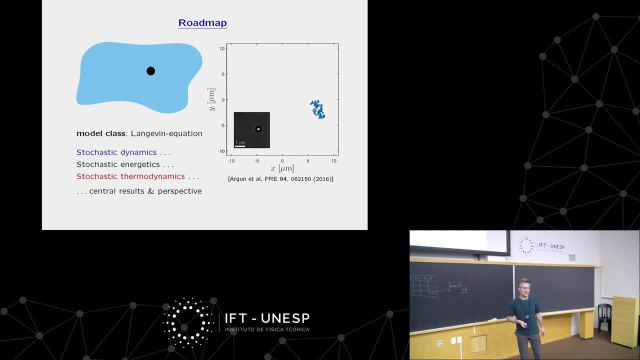 And this is an example for the trajectory you measure over a certain time. So it indeed looks like that, And the roadmap for my talk is that I focus, I will describe, I will describe these things, focusing on the model class of Langevin equations. 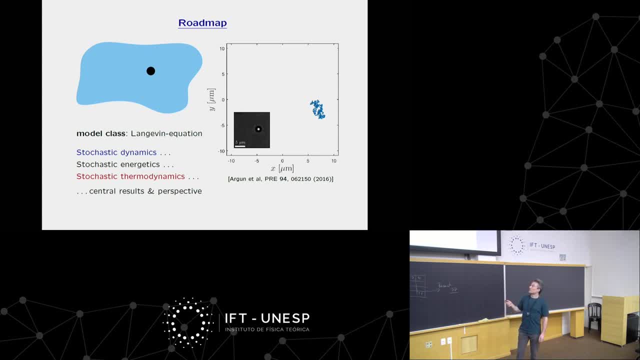 which are an extremely good model of this kind of systems, of this kind of motion. And then- this is very well known- the stochastic dynamics of these particles You learned already. it has been: The theory has been initiated. The development of the theory has been initiated by Einstein's paper 1905. 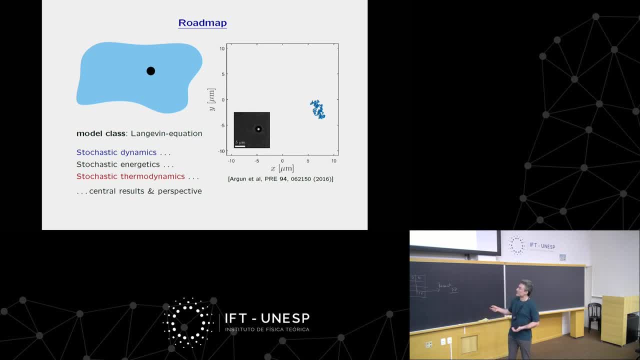 So it's over 100 years old, But these things, how you can do energetics with these systems, and even thermodynamics, this is a little bit younger. This is over the last 20 years. I would like to describe to you how this is done. 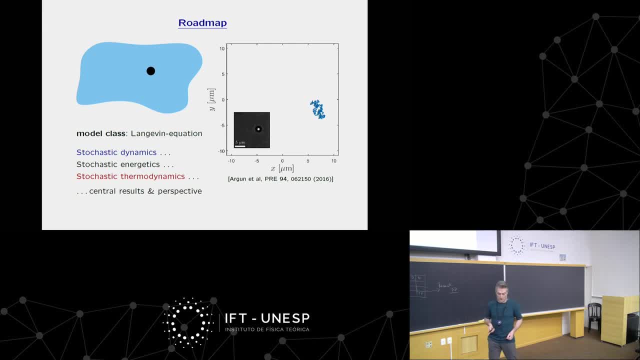 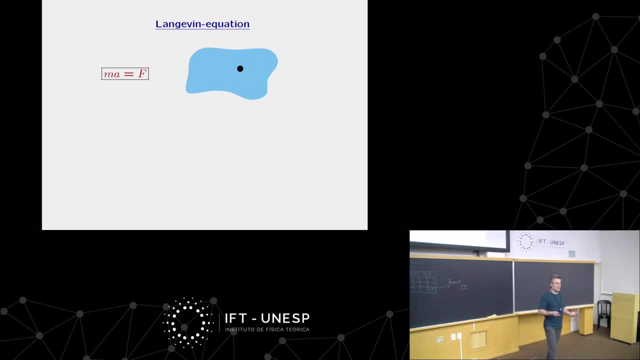 And then I will discuss a few central results and give a sort of perspective. This is the roadmap of my talk, So let's start with the Langevin equation. What we want is an equation of motion for this individual particle, where we include the effect. 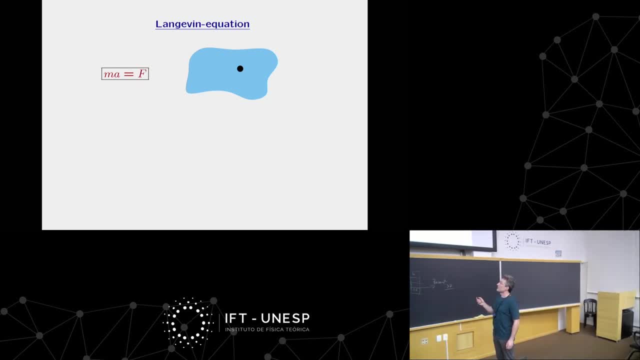 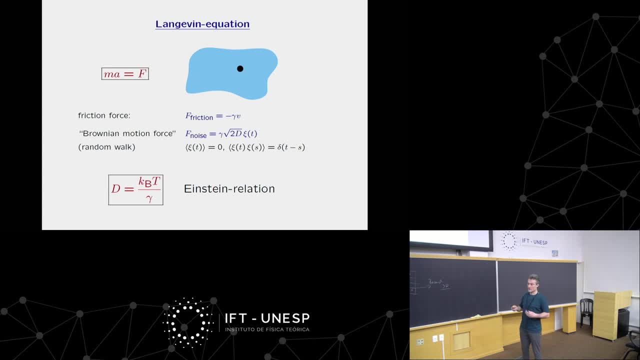 One is the friction. friction forces, That's the average effect of the bath, which is proportional to the friction coefficient of the particle gamma and the velocity, the actual momentary velocity of the particle. And then And then, the second effect is this Brownian motion force: 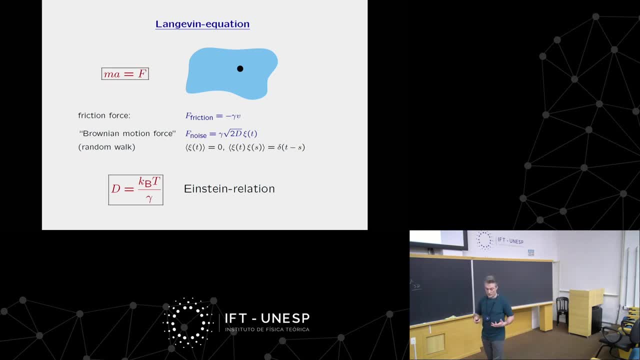 which is a noise force which creates this wiggling motion. So it's indeed modded by a random number And the most common model is a Gaussian noise. And if I say it's Gaussian, you know that I only have to specify the first two moments. 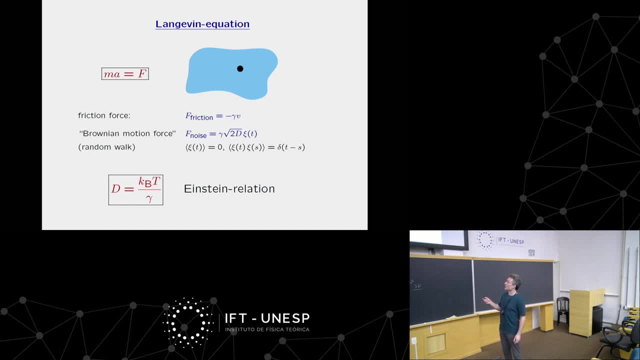 to fully specify the statistical properties of this object here. So the first moment is zero- There's no systematic component in this noise force- And the second moment is a data correlation in time, which says that the memory in this aqueous solution is extremely short. 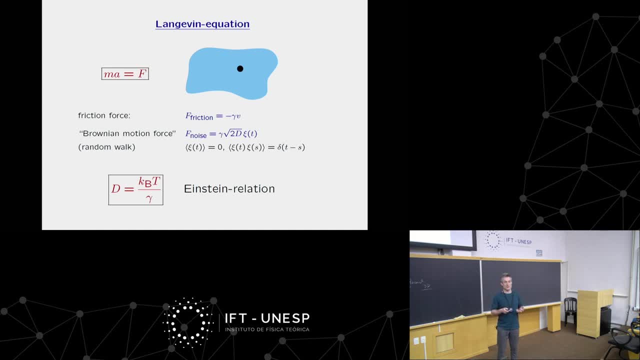 It's much shorter than anything else you're interested in, So that I can say that it's actually uncorrelated for any practical purposes. That is what the data function says here. And then we also know that this noise amplitude, the strength of the noise, must somehow be related. 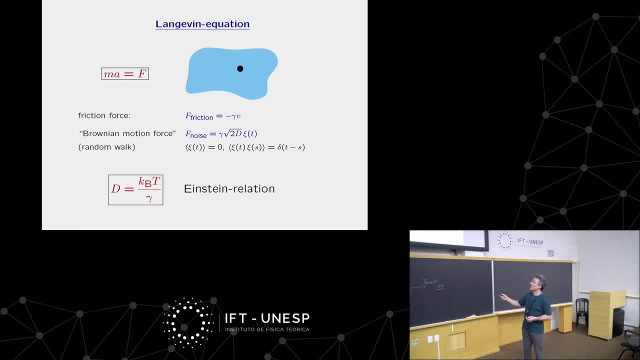 to the diffusive properties of the particles And, if you choose it like that, you recover what you know from equilibrium statistical physics when you calculate the distribution of the particle following from this dynamics. This is what we have seen in the lecture And Einstein found that this diffusion coefficient here is related. 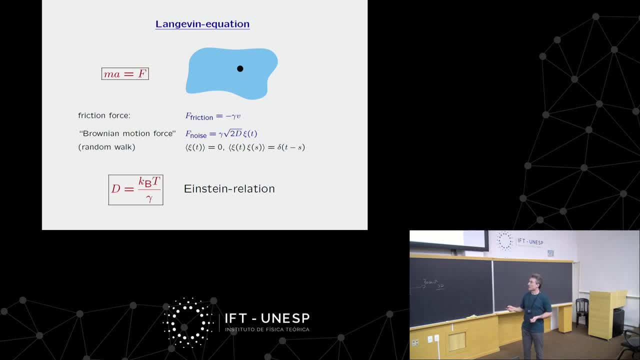 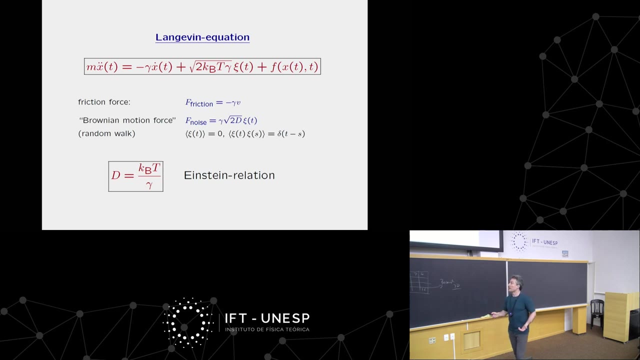 to the temperature of the bath and the friction coefficient in the particle in that way, And this is called the Einstein relation, And KB here is Boltzmann's constant. So we have these two forces which account for the effects of the bath, and then we can add other forces too. 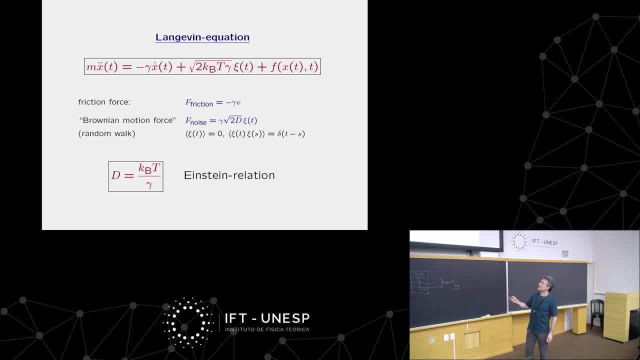 which I write here in this small F. So this is the full equation of motion. now For the particle, it's called the Langevin equation. MX double dot acceleration is equal to minus gamma X dot. This is the friction force velocity here. 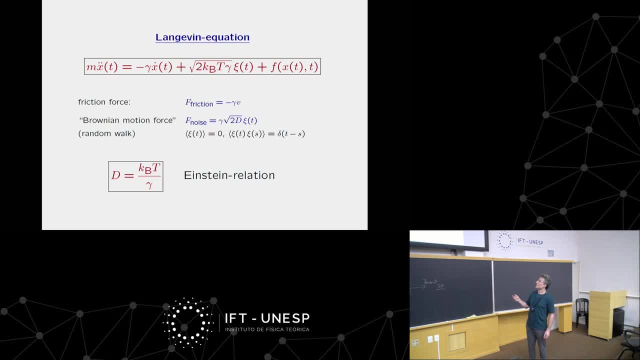 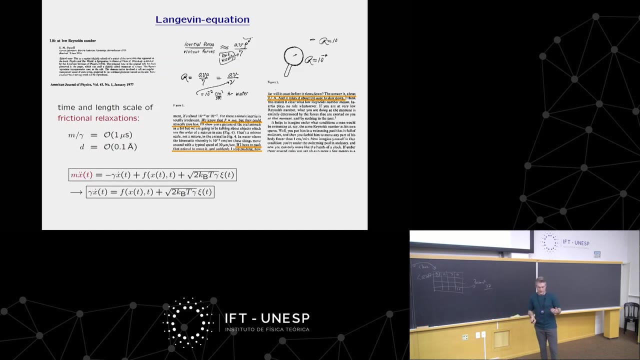 plus the fluctuating force, psi of T and other forces which are not due to the bath, like external fields and things like that. Okay, this is the equation of motion we're going to work with. And now I also mentioned in the lecture already: 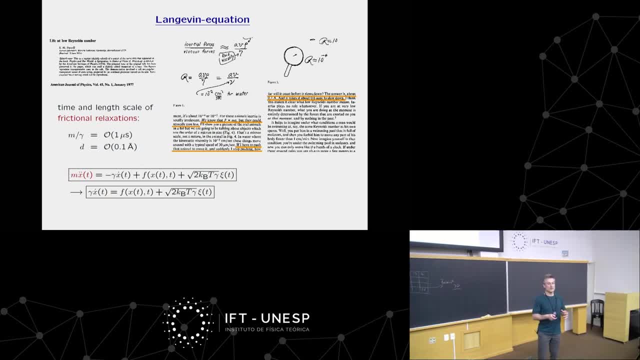 that X double dot. actually on these scales, on micrometer scales, even in water the motion is highly viscous And this is very nicely described in a paper by Purcell in 1977, where he says: we know that F equals MA, but they 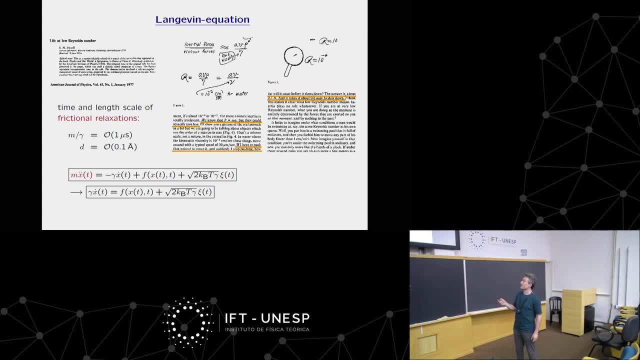 these objects he's also talking about, I think, bacteria, or so they could scarcely care less. If I have to push that animal to move and suddenly I stop pushing, how far will it coast before it slows down? The answer is about 0.1 angstrom, so less than the size of an atom. 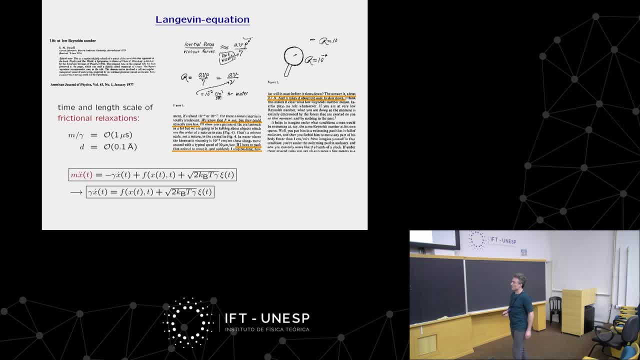 And it takes about 0.6 microseconds to slow down. So these time scales and length scales are also extremely fast, so that, again, for most practical purposes, we can forget about the inertial effects in this motion And we can go to the overdamped description. 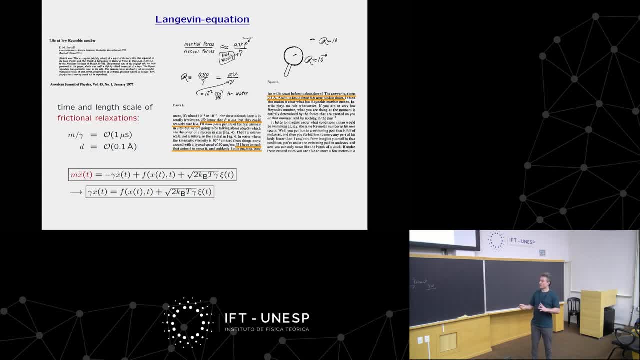 So, in fact, forget about this, set it to 0,, let's say, and end up with an equation which is first order in the position of the particle. Okay, And this is called the overdamped equation. This is what we have seen in the lectures. 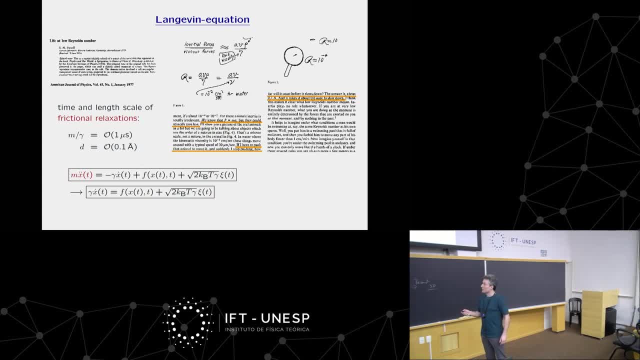 And, as I said there as well, this, what I described now, is a phenomenological way to get it, But this limit here, going from this description to this description, is mathematically tricky because you are dealing with a very complex equation. So, in fact, forget about this, set it to 0,, let's say, and end up with an equation which is first order in the position of the particle And, as I said there, this, what I described now, is fundamentally tricky. So, in fact, forget about this, set it to 0,, let's say, and end up with an equation. So, in fact, forget about this. set it to 0,, let's say, and end up with an equation. 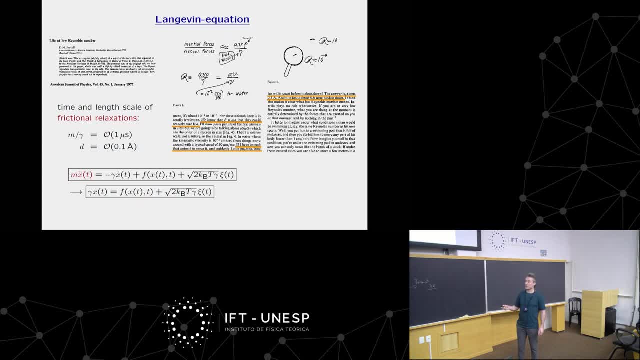 So, in fact, forget about this, set it to 0,, let's say, and end up with an equation, And you have to deal with the singular limit here, changing the order of the differential equation, and you have to deal with this weird object. 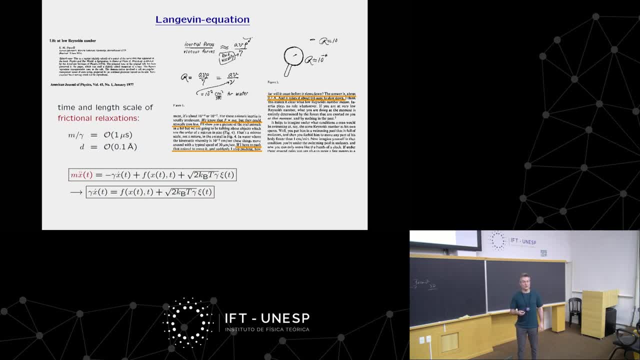 with this noise term which is in fact nowhere differentiable: continuous, but nowhere differentiable. So it's a tricky limit. If you do it carefully, you will, for most cases, end up with these equations. So we are fine here. 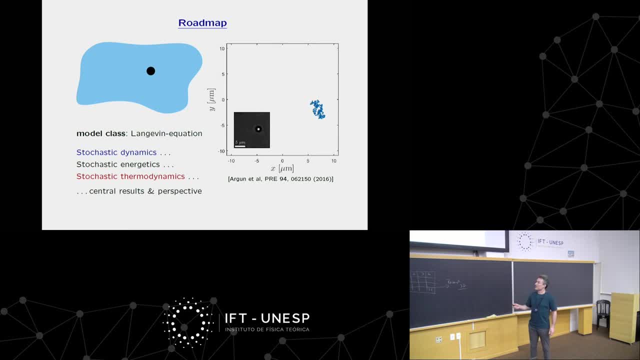 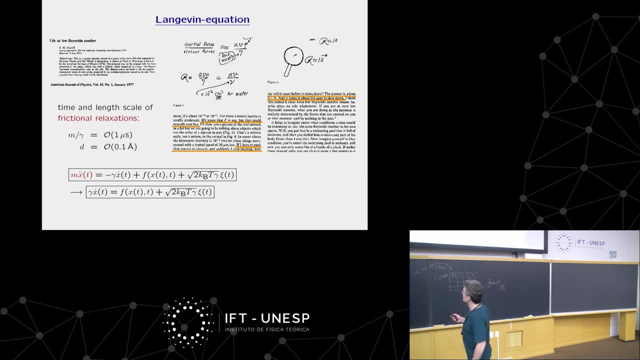 Okay, that's so much about the first part, the stochastic dynamics Compared to the friction. You compare m to the friction, So actually we are talking about timescales in the systems And this timescale- here m divided by gamma, is a timescale. 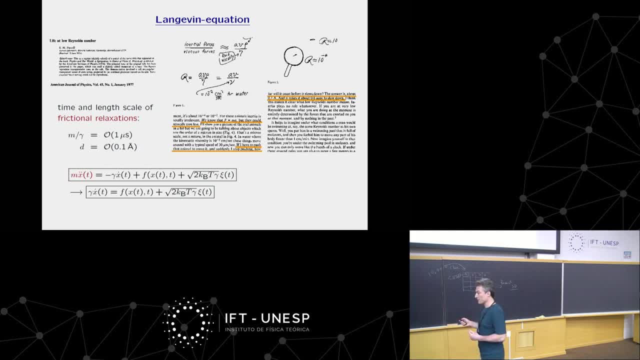 It's the relaxation timescale of the velocity degrees of freedom of the particle. I think he's confused because what he said is group of bacteria. it's not true for you. No, no. So when I mentioned the proper methods, bacteria have this sort of low rate of number behavior. 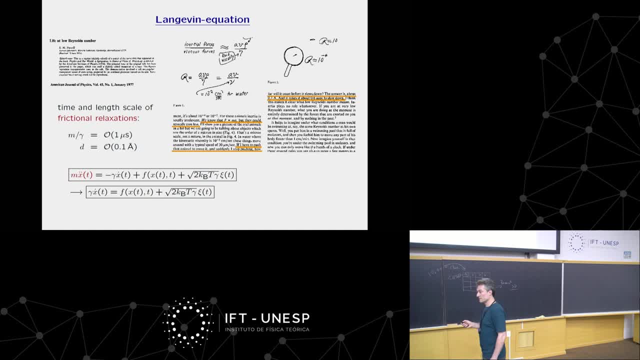 That's a good cell work, but you don't I understand. I'm just asking. so what's the parameter which has this model? m has units, m over gamma has units. Exactly, It's a timescale and you compare it to the timescale of the motion you observe. 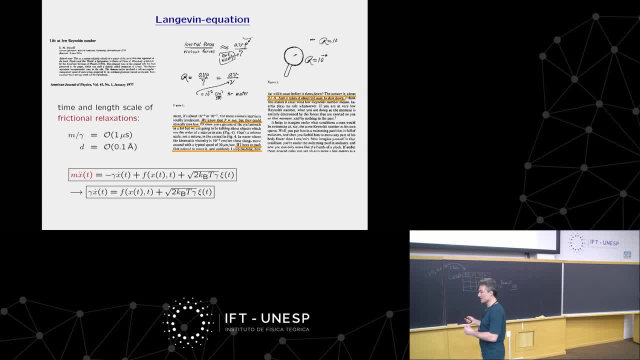 the diffusive timescale. Okay, Yeah, Good, And this ratio is about 10 to 6, or 10 to minus 6.. Okay, Actually, this model describes the system so extremely well that I met people who say, okay, I did this theory. 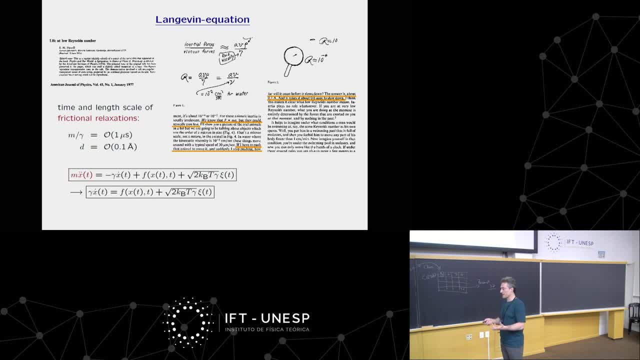 and then an experimentalist was saying: oh, I can measure that. and then the other guy said: why do you want to measure it? You know that it's working. So it's an extremely accurate description of these systems. Okay, Yes. 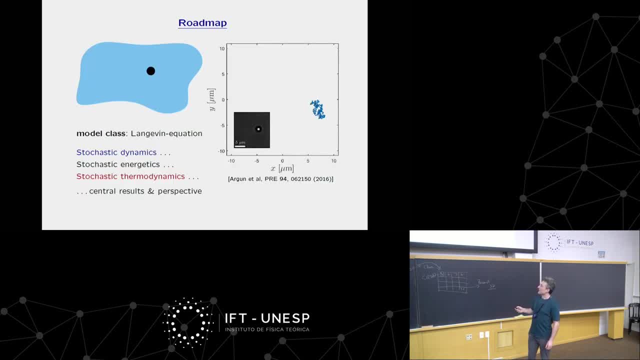 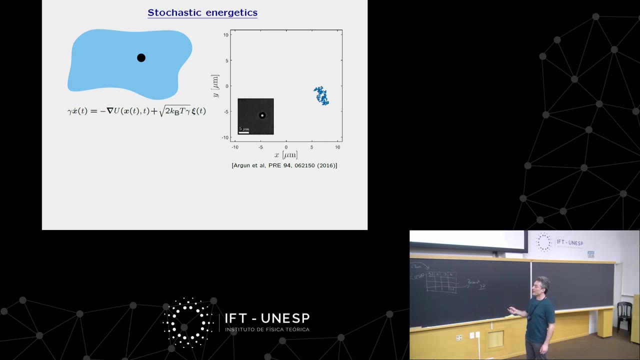 So far about stochastic dynamics, and now I would like to describe how you can do stochastic energetics with these kind of models. let's say- And I write down the Longer equation again, and now I consider the external forces coming from a potential. 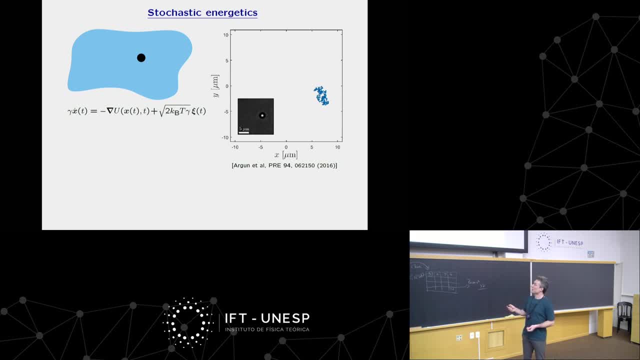 So this is a gradient of a potential u which depends on x, and I also allow it to be, And I also allow it to be, And I also allow it to be Time-dependent, explicitly time-dependent, And the idea here is that we are doing an experiment. 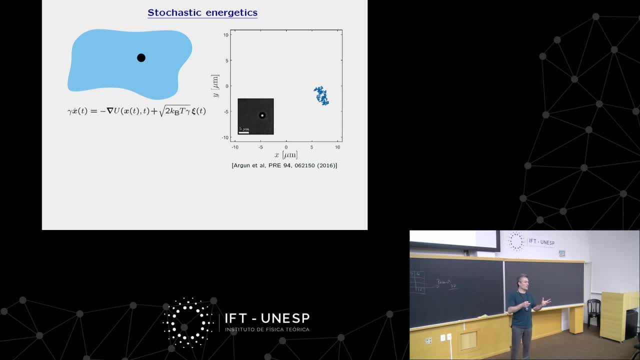 Imagine a colloidal particle, for instance, or a protein or whatever your favorite small particle is, and you say you use a laser, an optical tweezers, to trap this particle and then you can manipulate it. You can change the laser intensity to widen the trap. 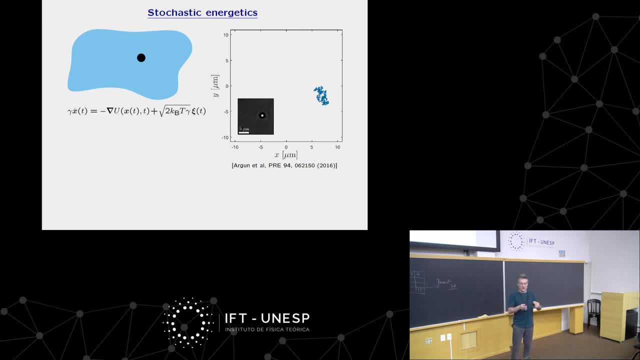 or increase it to narrow the trap. You can move the particle, And this is something The experimentalist does. So he does some adjustments with his equipment and this changes the property of the system. This is like an external control parameter. you have to manipulate the systems. 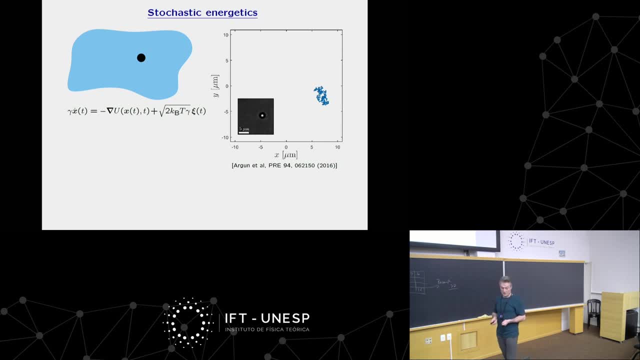 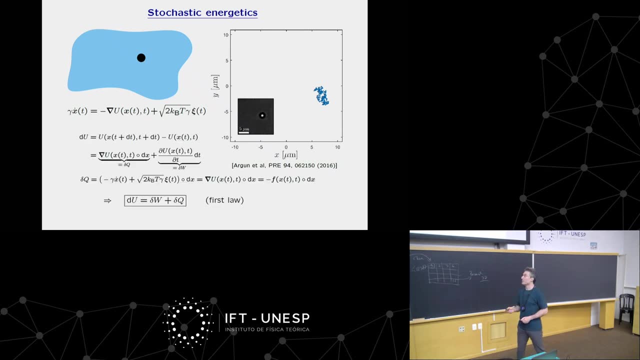 And this is hidden in this explicit time-dependence of the potential. Okay, This is what we mean here. So now I look at the change of the potential energy. for a small step the particle does, and then a time step, dt, So it changes position from x of t to x of t plus dt. 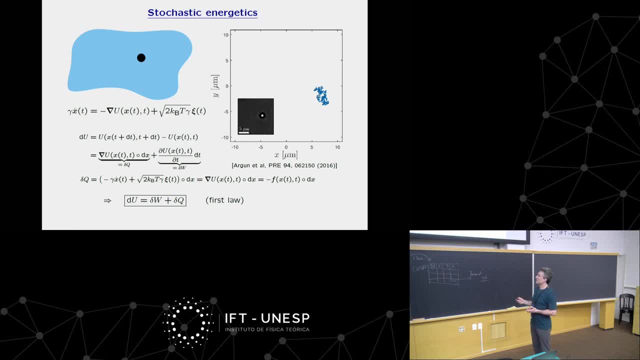 And then the energy changes too here, due to the change of position and due to maybe some external changes. And if I expand this I get two contributions: gradient u times dx and du, dt times dt. And now I have to interpret these two contributions. 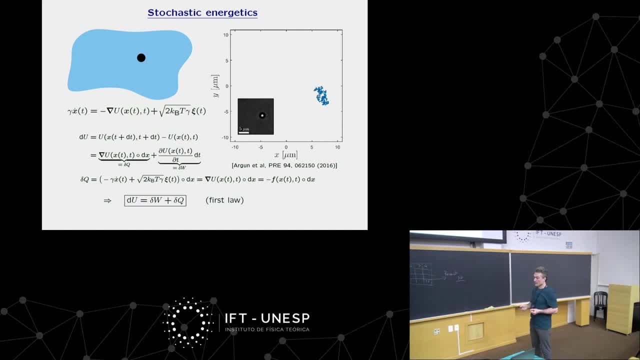 And for the first one, we look at this equation. If I want to talk about heat, what is heat in that system? Heat is the work exchanged with a heat bath. So the forces, the particle exchange, or the forces that act on the particle from the bath times, the displacement, 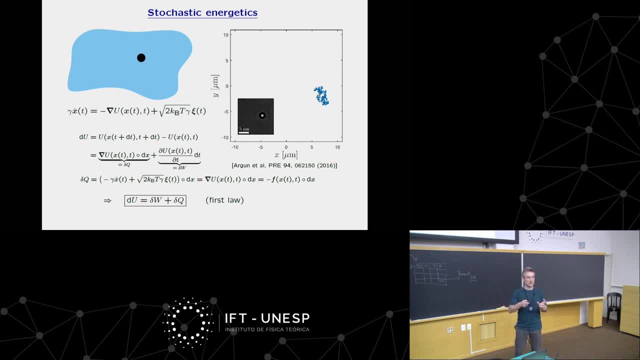 This would be the energy. the particle exchanges with the bath And the energy. Since this is a heat bath, it's heat by definition, And this is what is written here. This is the two forces that come from a heat bath, right from the solution. 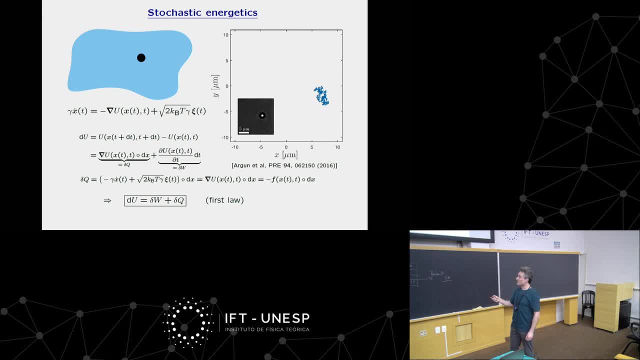 friction and fluctuations, times, dx, times, the displacement. This gives you heat, And now I use the equation of motion to replace this part here by the gradient of u. It's just the balance of forces I use here, And I end up minus u. 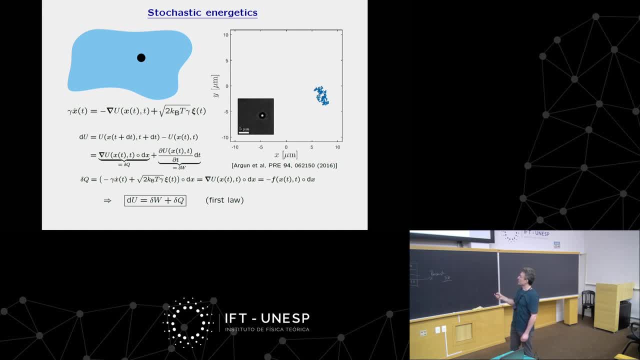 And I end up minus u, And I end up minus u. Minus u is minus gradient, u is minus f, So that this contribution here is actually the heat, the particle exchanges with the bath. Okay, And the second contribution, this is a change in the energy. 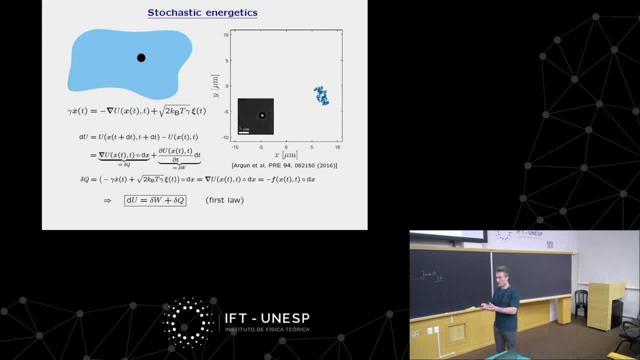 which is due to external manipulations. So you mentioned, the particle would not change its position, but the potential is changed by the experimentalist. Then still, it changes its energy constant And this is what people identify with work here. So this is the external work. 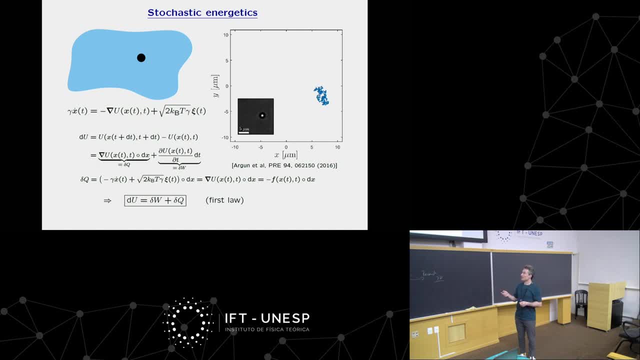 And then we see that du is equal delta q plus delta v And we have a first law for this step of the motion of the particle. So this is the first law: a balance of energy flows in the system. Okay, And of course you can integrate along the whole trajectory. 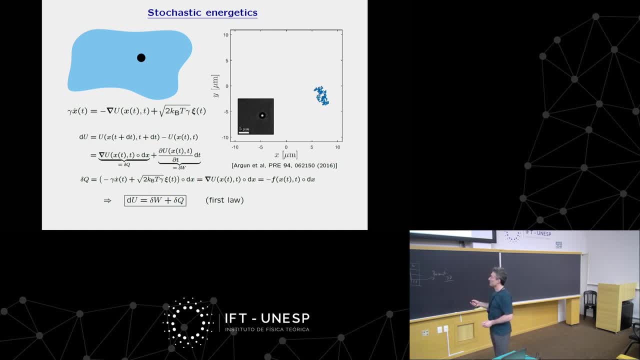 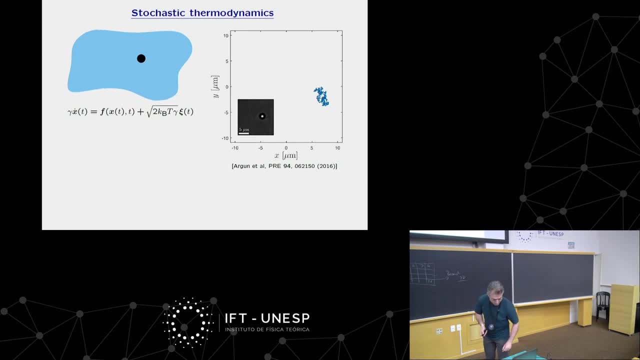 and get the change of energy as a complete work along the trajectory and the complete heat exchange with the heat bath. So now this is energetics. But what about stochastic thermodynamics? What about thermodynamics And thermodynamics? I started with a second law. 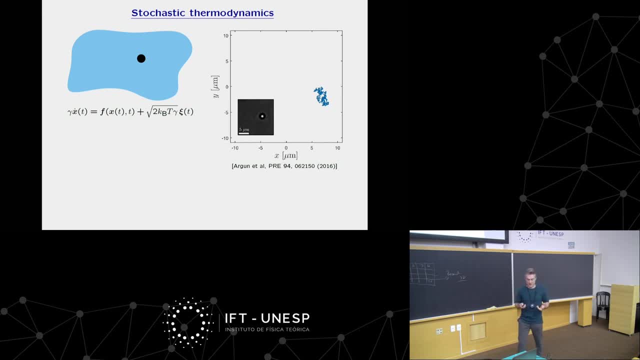 What we want somehow is we want to quantify entropy, And is this possible? The idea here is to look at the following situation: We are thinking not yet about entropy, But we ask the question: how irreversible is that motion? So you know, these movies you see sometimes. 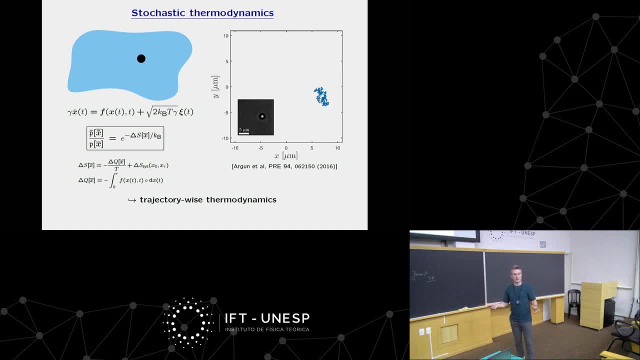 The cup is falling from the table and breaks, And then it's not, And then it's not, And then it's not, And then it's jumping back on the table. When you see, it's jumping back on the table and reassembles. 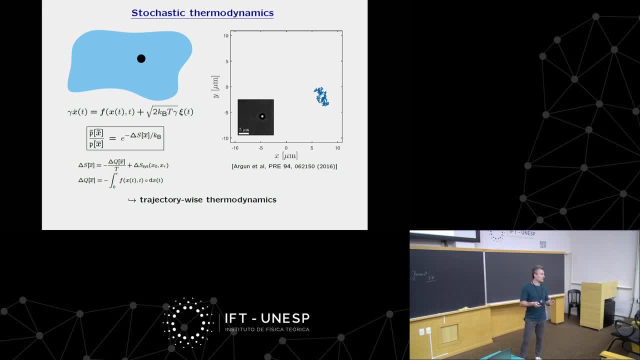 you know you have seen the movie running backward in time. Okay, Because you know from experience that such a process has never been observed in reality? It's extremely unlikely. And here we ask the same question for the system. We look at the trajectory. 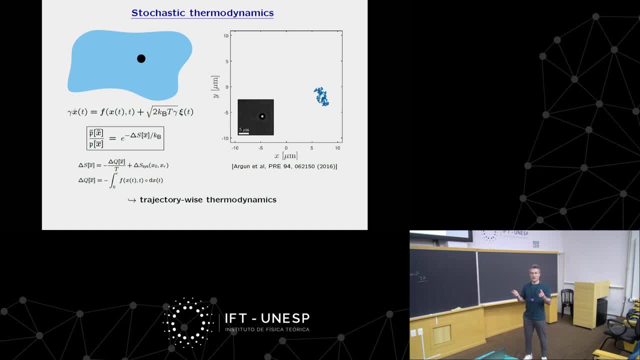 this trajectory, which has been measured in an experiment, and we ask the question: how likely is it to, how likely is it to observe exactly the same trajectory, but traced out backward, backward in time? This is what I've written here. This is the probability of the trajectory observed forward in time. 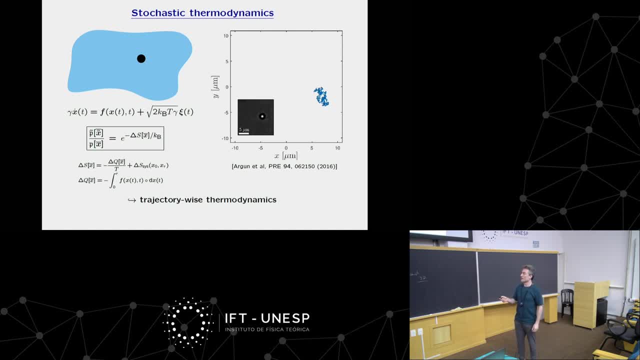 So this X bar collects all the positions of the particle along a certain trajectory, compared to the probability of observing the same trajectory, but traced out backward in time. So we try to quantify how irreversible this is, How irreversible the dynamics of this particle is. 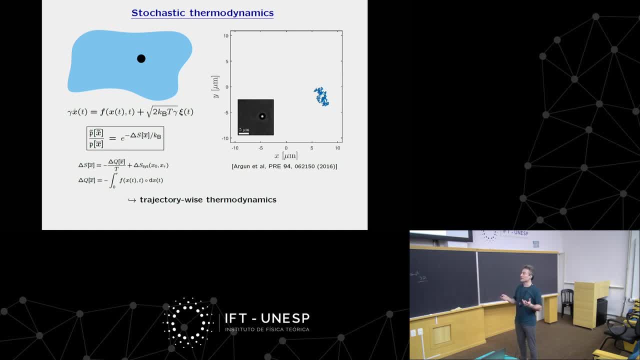 And then I find after some calculation which involves path integrals- I don't want to go into details- that this can be written that way. So now I wrote it already very suggestively here- the delta S, And this delta S is actually this quantity where this delta Q divided. 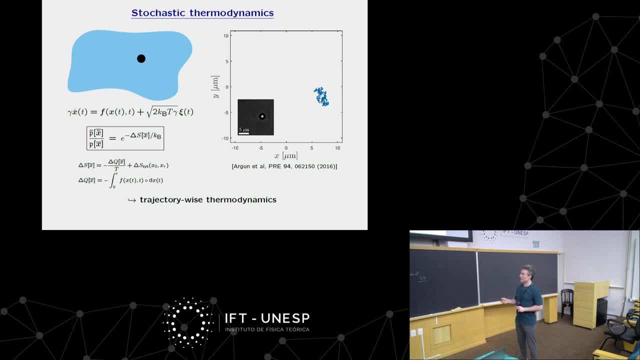 by T here is given by the term we identified earlier, by the heat, the particle. So this is the heat that the particle exchanges with the heat bath And this contribution here is called the entropy production in the medium. So I repeat, this is the heat the particle exchanges with the bath. 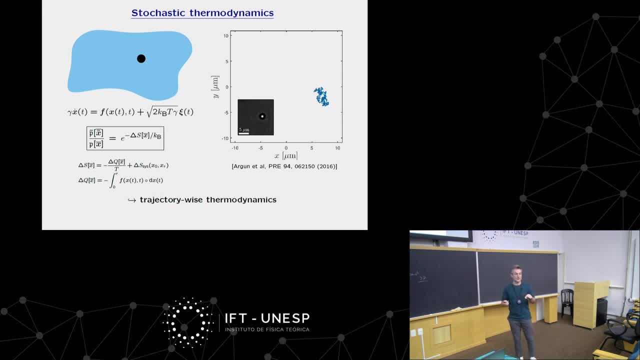 and this corresponds to a change of entropy in the bath. Okay, And this is this quantity here And this part here is the contribution of the boundary initial and final position of the particle which you can identify with the entropy of the system. 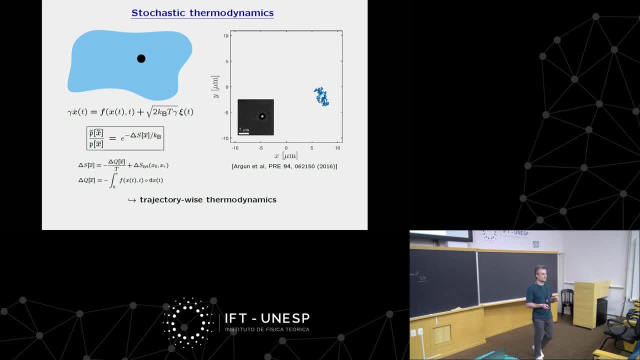 So with the entropy of the particle itself. So we started here from a different question. We asked a question of irreversibility and have seen that this question is answered actually by what we naively would define as entropy from this motion of the particle. 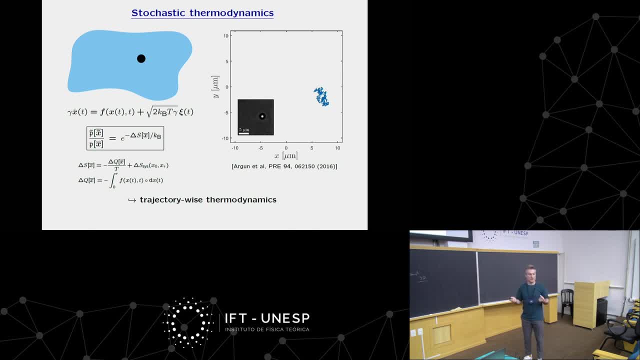 or which is actually an entropy change in the bath. The irreversibility of this motion, how likely it is to observe forward versus backward changes, is connected to the entropy, which is like dumped into the bath. you can say, Okay, This is one of the main results of this approach. 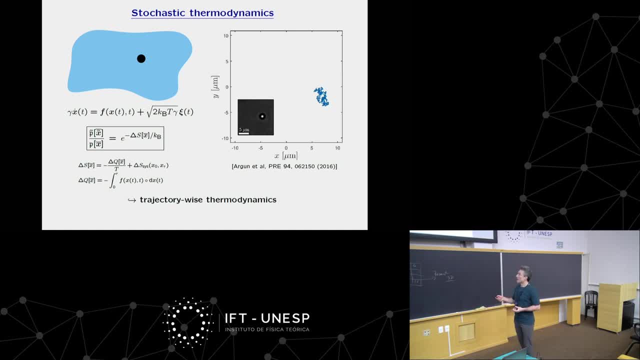 And this is the essence of stochastic thermodynamics in a way, And a better name may actually be trajectory-wise thermodynamics, because you look at all these quantities along trajectories, so along evolution in time. The term stochastic thermodynamics is a little bit different. 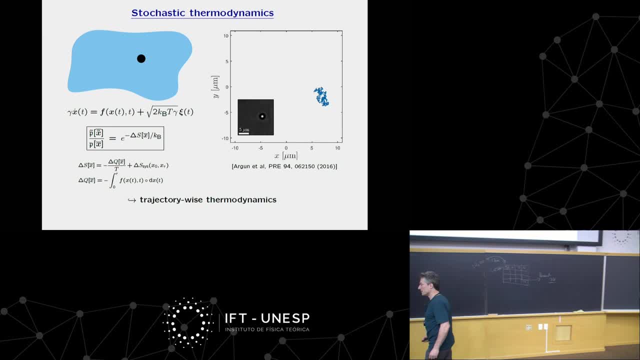 It's a little bit historical. Yeah, I don't know if this is supposed to be rigorous, but how do you define T of X-parts? And you have to know all the trajectories. Yes, yes, How do you possibly do that? 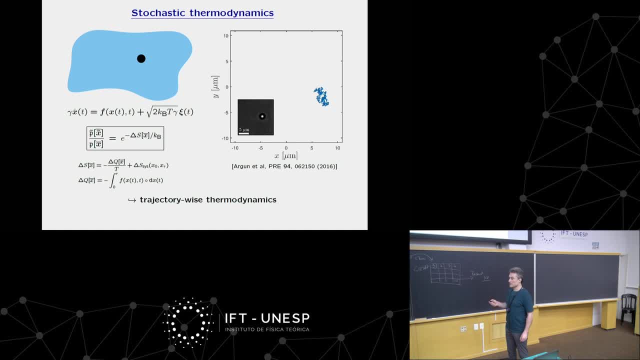 You can calculate this by using path integrals, So you're very similar to quantum mechanics. You write, you discretize this equation and write it, and write the probabilities for the single steps and from that you construct the probabilities for the whole trajectory. 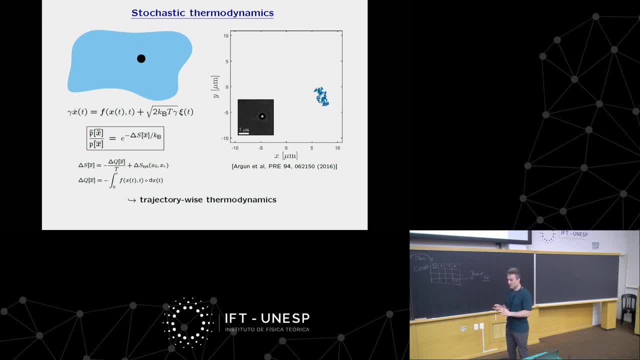 And these you can write down up to an unknown pre-factor, but it cancels out. an unknown pre-factor which is independent of the trajectories, but this cancels out if you take the ratio. So just a couple questions. Okay, This is fine because you have a best constant. 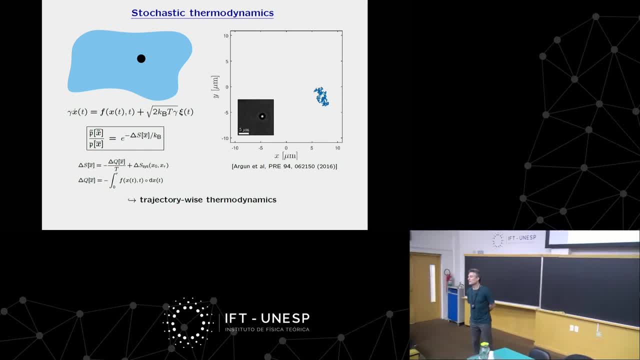 of your temperature and gamma. Yes, How do you compute the delta S system? Do you have an expression for it? Yeah, It's the ln P of X minus ln P of Xt, basically. So it's the ratio of the logarithms of the probability. 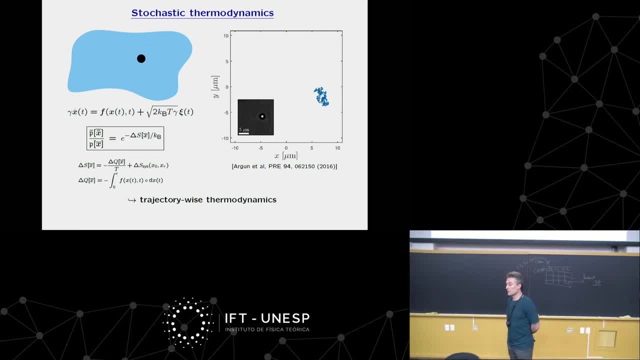 What's P of X0 and P of Xt? The probability of the system coordinate at the beginning and the end of the process. How do you write that? I'm trying to figure out what the expression is. If you don't know what I know, how do you write it? 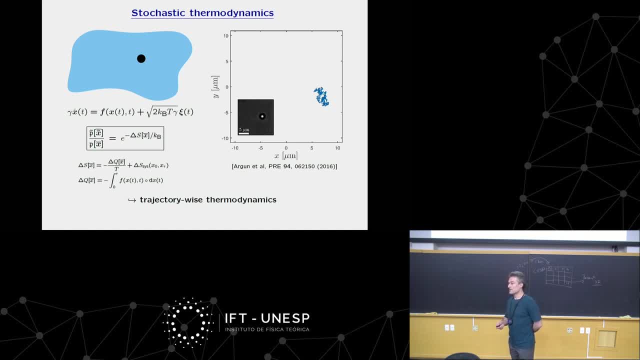 No, it's So. P of X0,, if you like, can be specified by the experimentalist. You can start your experiment in. You prepare your experiment in a certain way and this gives you how likely it is to find this particle. 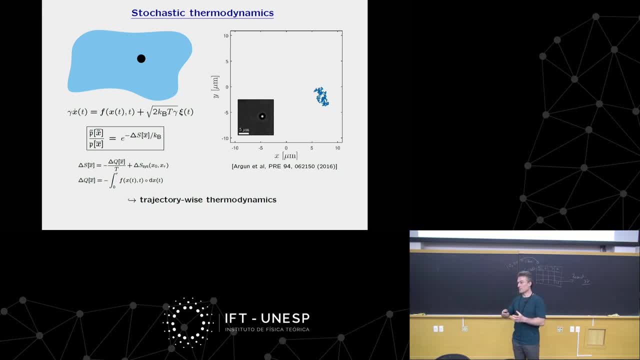 you're manipulating at a certain position And the P at the end of the process is that which comes out as the probability when the particle evolves, with the Lausanne equation, Or, for the probability densities, it's the Fokker-Planck equation which is. 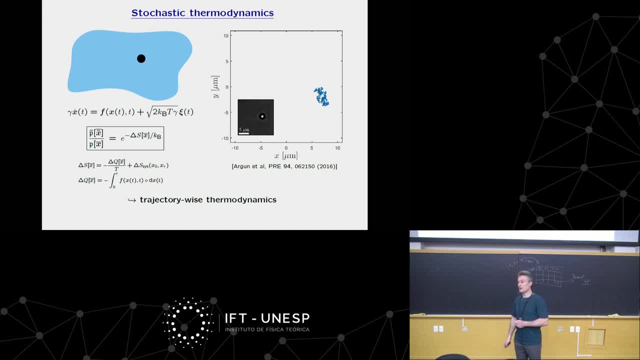 No, it's the usual time evolution. You don't have a path integral for that, Or you can get it from a path integral if you like, But you have to compensate from the best right. So it's not like you're X or P. 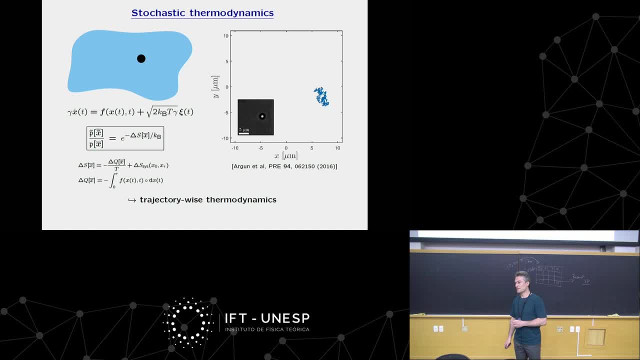 It depends on the best right. Uh, no, no. So if you put P of X0, let's assume you have an experimentalist, you have an optimal three-dimensional equation and you have an experimentalist, you have an optical tweezer. 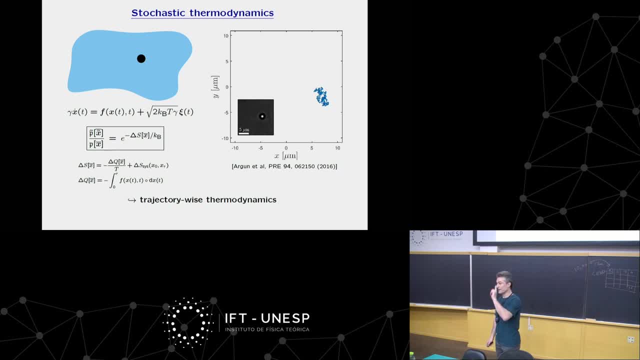 So I put: P of X0 equals 1. Right Or delta. yeah, Now I can evolve or make a different thing, but that may depend on the best. Yeah, that's what I say. This P of Xt which enters here: 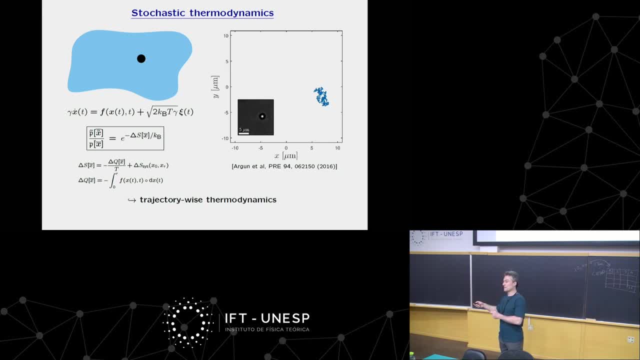 is the one you get from the evolution of the system, And this is Yes, yes, sure, sure, yeah. It's a distribution. Yeah, Um yeah, But it's a boundary term, So often these things are written down. 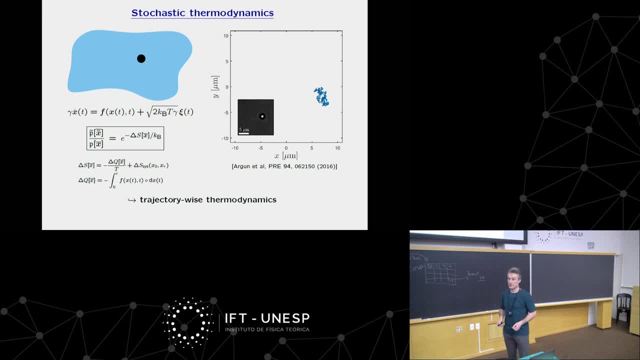 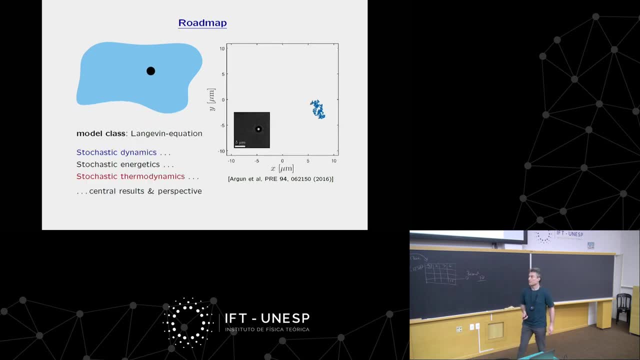 without the boundary term, because for large times they don't play a role anyway. Okay, Uh, yeah, So We're already here. This is what I want to tell you about the stochastic thermodynamics. So how thermodynamics become stochastic in these systems. 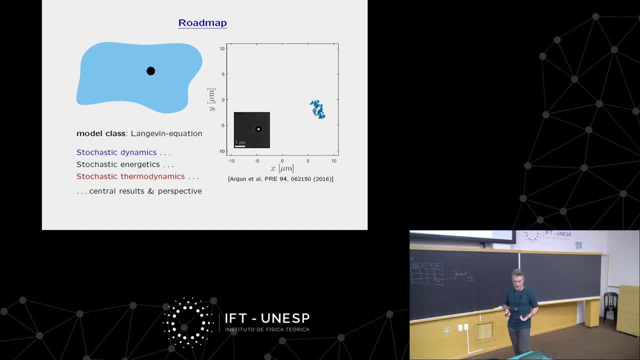 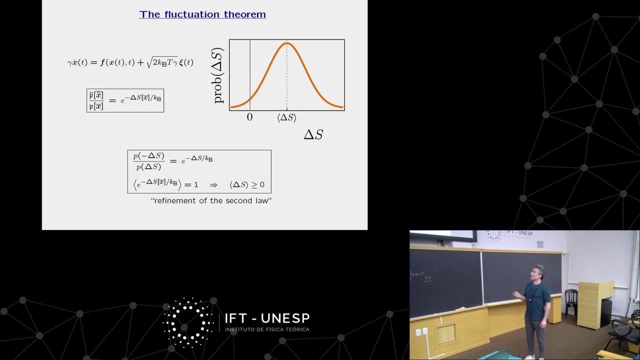 And now I would like to list a few central results which have been derived with these kind of approaches and which I think are very interesting, And the first one is these fluctuation theories. So we start with that, We get this here And from this probability of the path, 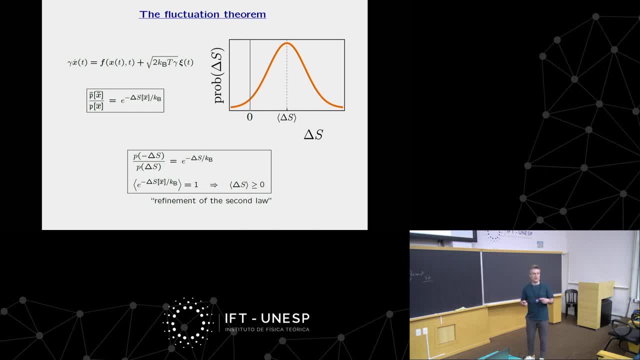 we can actually calculate the probability of observing specific entropy changes. and the probability of observing a sort of negative entropy change compared to the positive one is given by this equation here. This is called a detailed fluctuation theory for the entropy production along a certain trajectory. 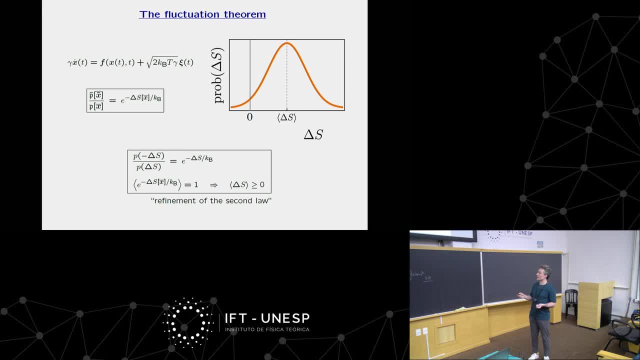 And then you can obviously average this here by bringing this on over the other side and average over all the pulses, And then you will get this expression And by the properties of the exponential you can directly derive this result from this here. So this is very often called 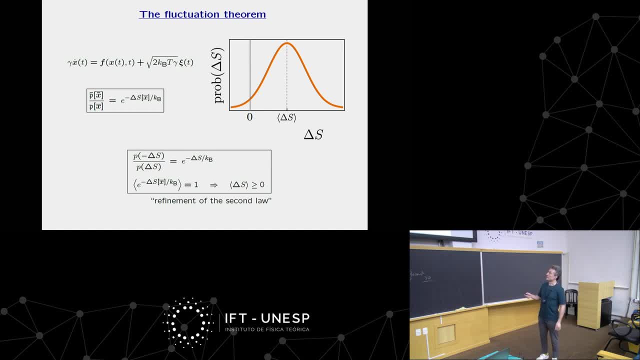 a refinement of the second law And it tells you that the entropy production along certain processes has a distribution, of course, because of the stochasticity, And sometimes this entropy production can even be negative, So people also call that sometimes transient violations of the second law. 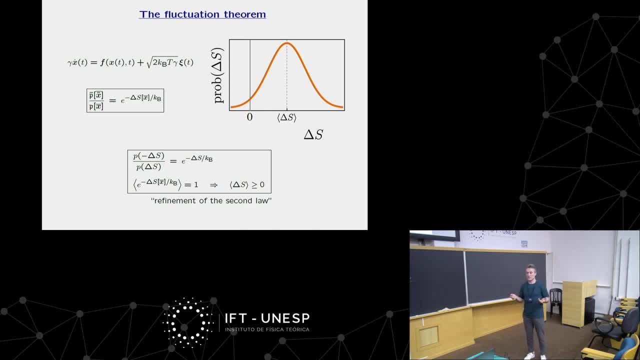 or things like that. But it's not really a violation of the second law, because the second law does not apply to these kind of systems. These are driven systems, so they are out of equilibrium. The system does not equilibrate with the heat path in these processes. 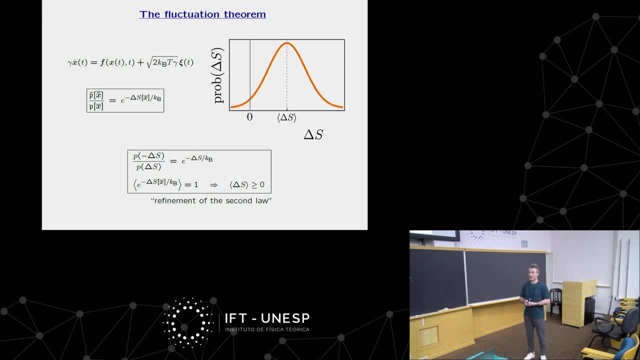 So with certain probabilities you observe negative entropy production, But the average here is always non-negative. This is the result which you also get directly from that. This is one of the results, And the second one, maybe the most famous one, is the so-called Sharzynski relation. 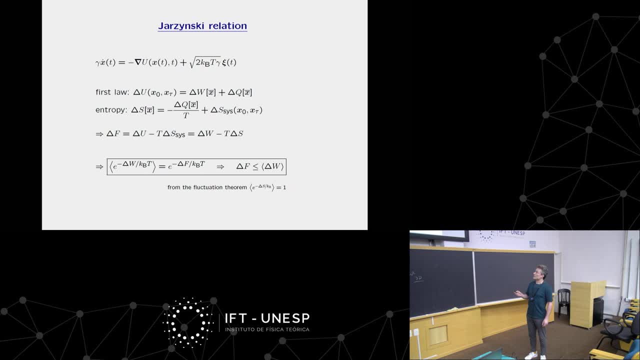 where you use these results. The first law: now I write it as changes in energy and work and heat along the complete trajectory And here's the entropy. And now I define a free energy which is given by the standard expression And then from the fluctuation theorem. I got here. 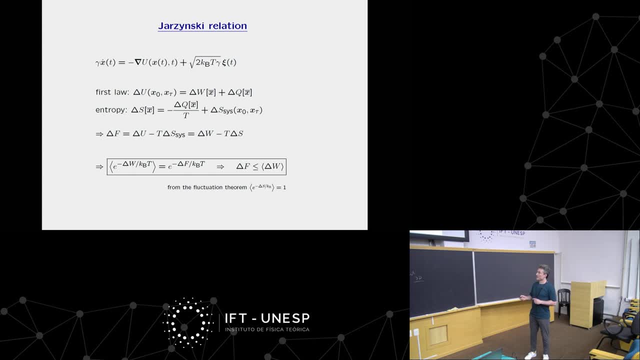 I get this result here, that E to minus delta V, the work averaged over many realizations, is the same as E to minus delta F divided by KBT. So what does this tell us, this relation? It says we do an experiment. 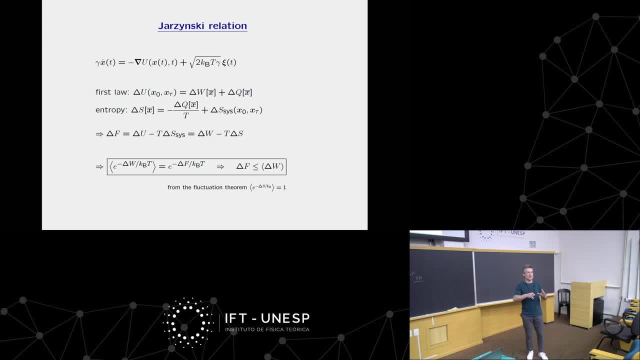 we prepare our system, we do an experiment, manipulate it in some way, measure the work we have to perform on the system to get this manipulation, or which we get back from the system. maybe It's a distribution of work And then we average this exponential. 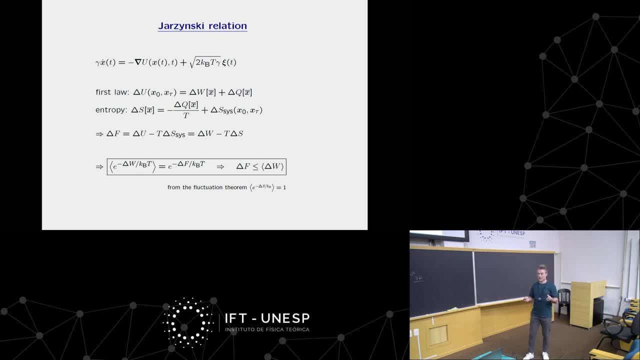 and we get a relation to the difference between the free energies of the system at the beginning and the end of this process, which is an equilibrium concept. So the system, when equilibrated with a heat bath, has a certain free energy at the beginning and at the end. 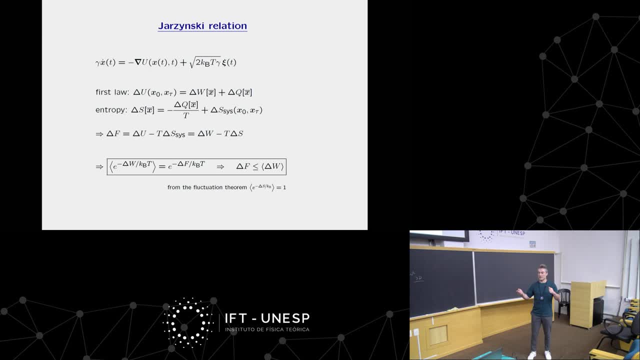 But in the middle between these beginning and end states, which are equilibrium states, the system can be far away from equilibrium. So this work I measure here is a quantity which is a non-equilibrium quantity, And the non-equilibrium measurements here are related to equilibrium properties of this system. 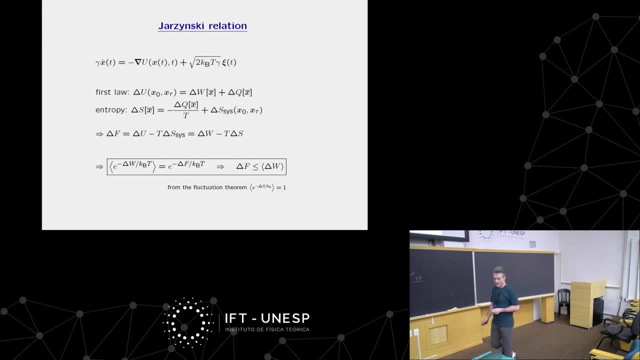 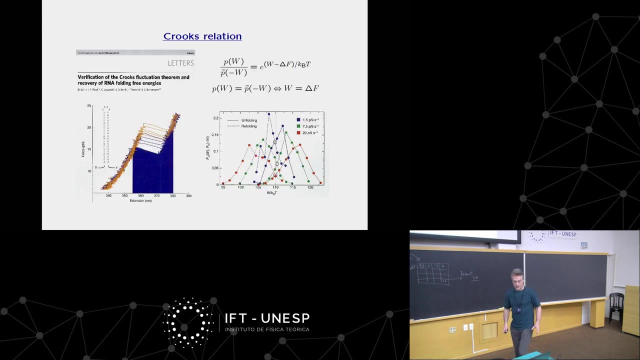 And this is a very famous result in that field and has been also tested experimentally, And it's very famous by now. And I will not present experimental tests of these relations, but another one which is very closely related, which is about the distribution of the work itself. 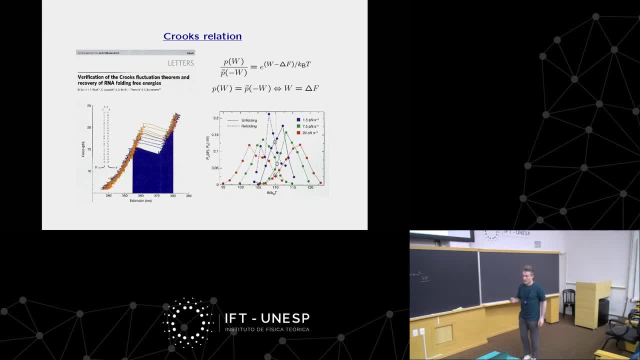 It's called the Crookes relation or the Crookes fluctuation theorem, And it says that the probability of observing a certain work which you perform on the system or which you get out of the system, compared to minus the work when you perform the same experiment. 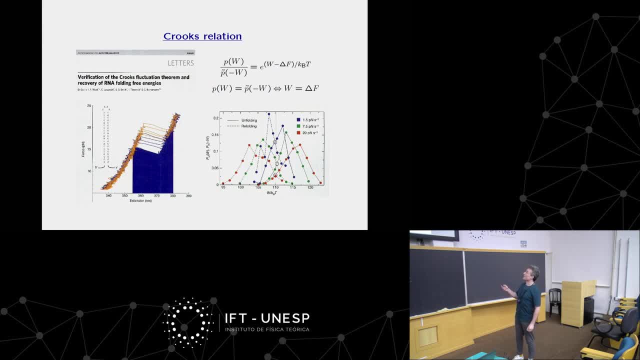 but with a backward protocol. Then it is given by E to W minus delta F divided by KBT. So here's an example. You have an RNA hairpin which is folded. This is this thing here. You connect it to a colloidal bead. 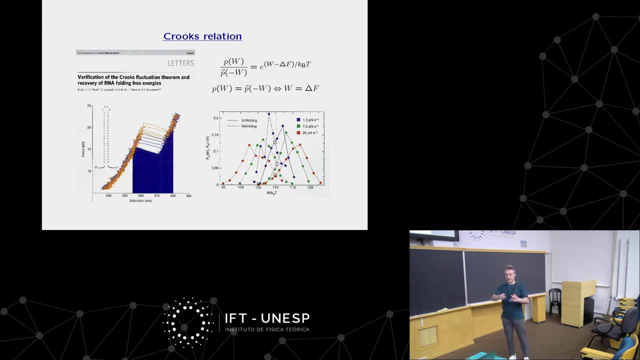 which is trapped by an optical tweezers, And then you can pull this hairpin until it unfolds. These are these curves, The orange one are the unfolding experiments. So it's this extension versus force And you see the fluctuations which are due to the thermal fluctuations. 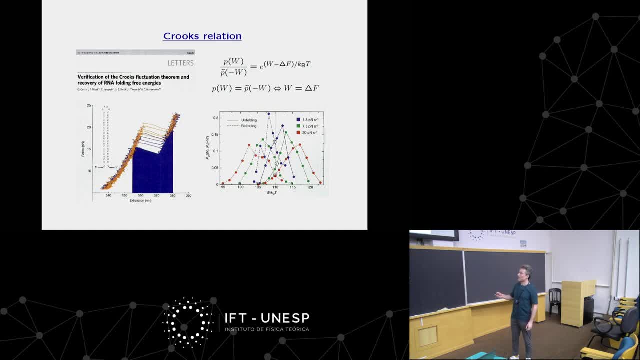 It's moving here unfolded, and then you perform the same protocol backwards, So you move your optical tweezers backward, And then at some point the hairpin refolds and gets back to its original state. And this experiment you repeat many, many times. 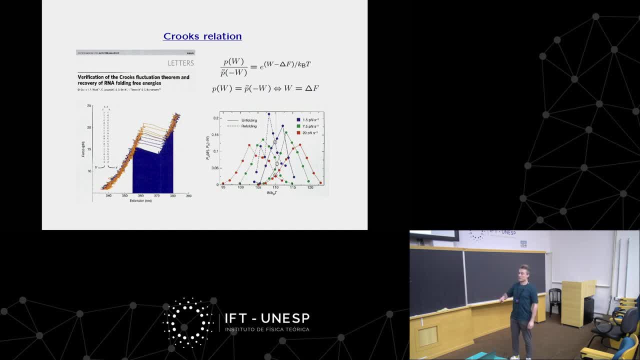 You get a distribution of the work in both directions. So here in this blue area, for instance, is the work which the system gives back to your machinery during one of the refolding processes. Okay, So you do this measurement: Measure the distribution of work. 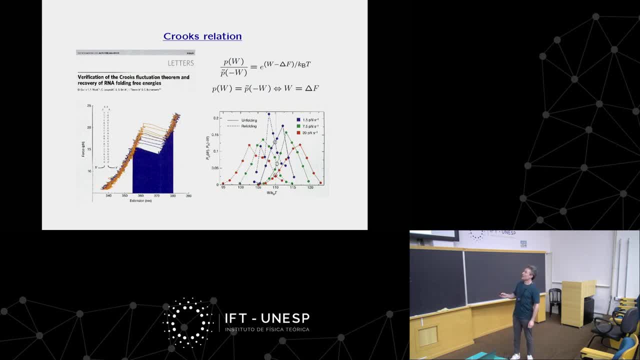 forward process and backward process and compare the distributions for various extension rates here for various protocols. It's the different colors And you find these curves. The dashed ones are the refolding experiments, where they plotted minus the work to get positive numbers, And the solid lines are the unfolding experiments. 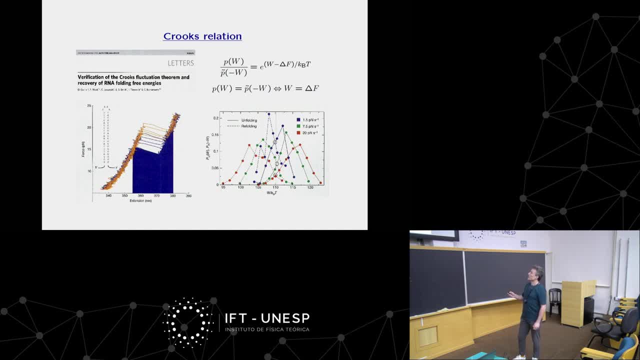 And this relation tells you that when these two probabilities are the same, the forward and the backward, then the work you performed on the system equals the difference in free energies between the folded and the unfolded state. Okay, And you see here, this is the line. 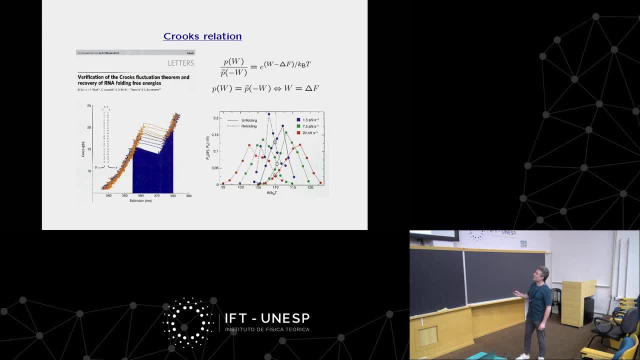 So this is the line where all these curves, within the experimental uncertainties, where all these lines cross. You see, the blue dashed line crosses with the blue solid line. So this is the point here where the refolding distribution equals the unfolding distribution, And the same for the green curve. 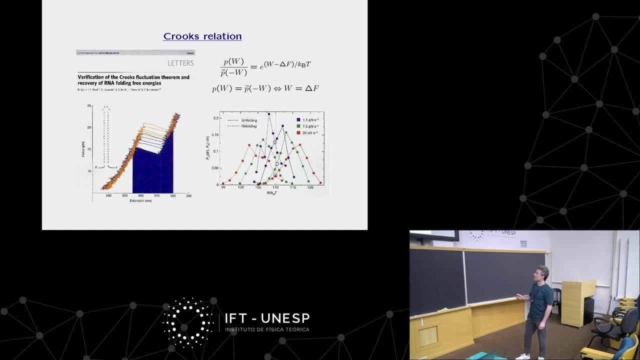 where you pull with a different rate and the red curve. Here's the crossing line. You see that this point here is independent of the protocol, which is the prediction of this fluctuation theorem, because it says: no matter what the protocol is, you can do what you like. 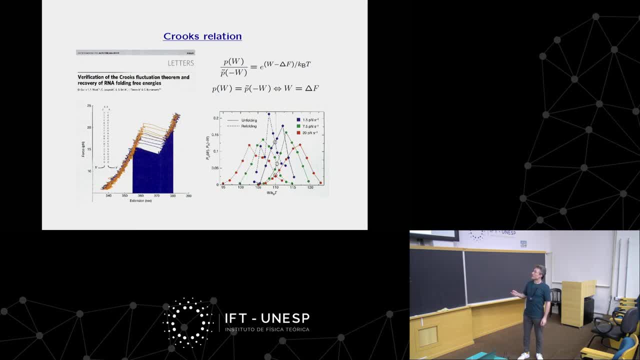 you will always find this relation And from that they got what the free energy difference of the unfolded versus refolded state And it fits very well to independent measurements for the other methods. This is just one example. It's one of the very earliest examples. 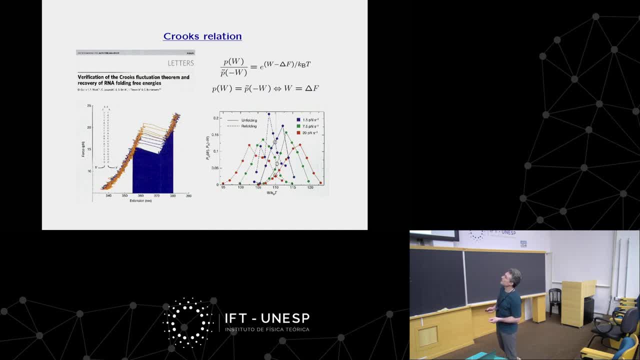 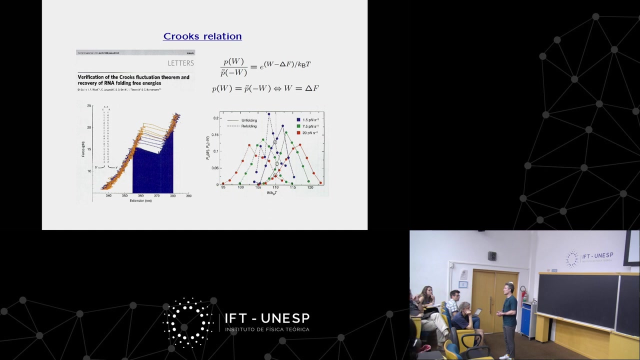 I think you can see 2005, maybe, or something like that, But there have been many more measurements by now. Yes, Sorry, No, you have to make sure that your initial and the final states are always the same. 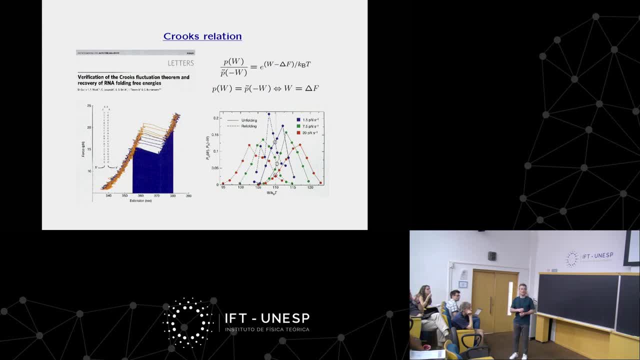 Yes, So the path in between will be different. It unfolds at different accelerations, At different extensions, But the end state has to be always the same, the same unfolded equilibrium state. Does that answer your question? Okay, Okay, good. 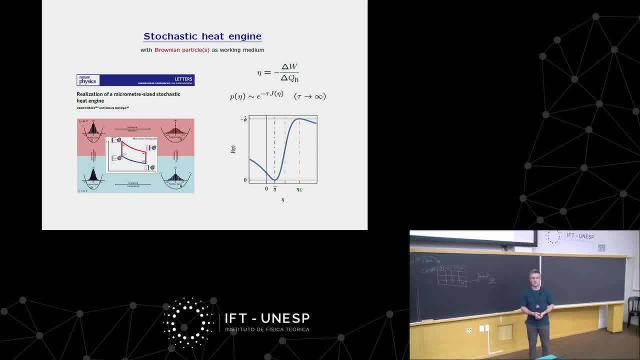 And then there are also applications of these concepts to stochastic heat engines. So this is also something like in your cell: there's energy conversion going on all the time And there's thermal fluctuations, So these can be interpreted as being stochastic heat engines. 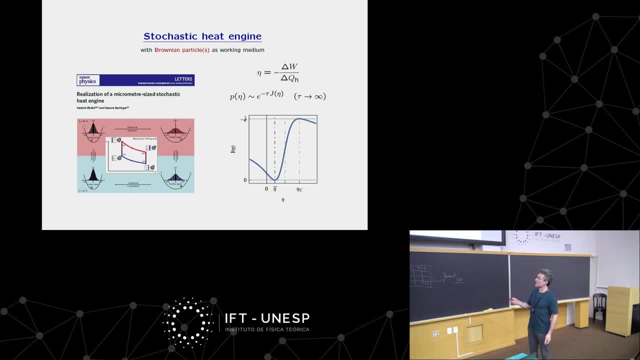 And people also build artificial ones, like this example here, where you have a colloidal particle, a Brownian particle, as the working medium for your heat engine. So you manipulate a Brownian particle which is trapped by an optical tweezers. 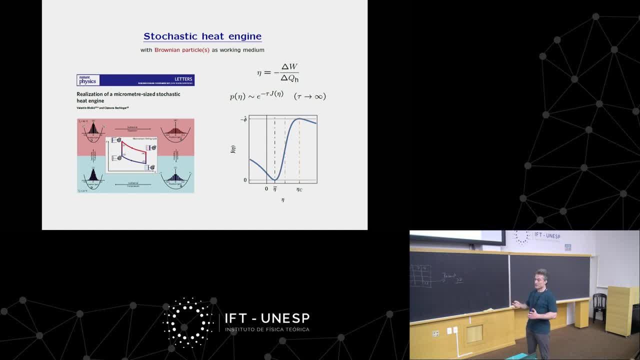 And then the expansion corresponds to widen the optical tweezer And the compression corresponds to increasing laser intensity and narrowing the optical tweezer, the potential here. And then you can heat and cool, So you get a cycle right And you can again. you can measure heat and work. 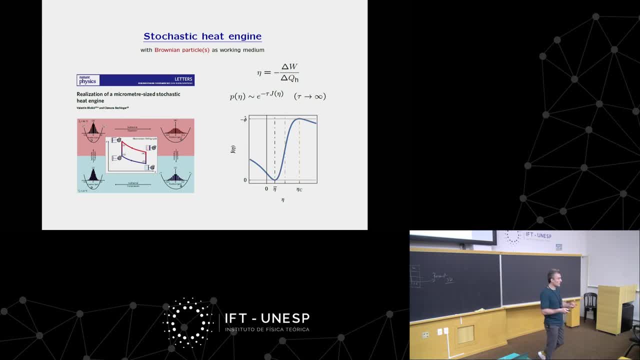 heat exchange with a hot bath or with a cold bath. you can measure the work and so on, And you can define an efficiency here, And the efficiency is defined as usual. It's the work you get out of this process, divided by the heat from the hot bath. 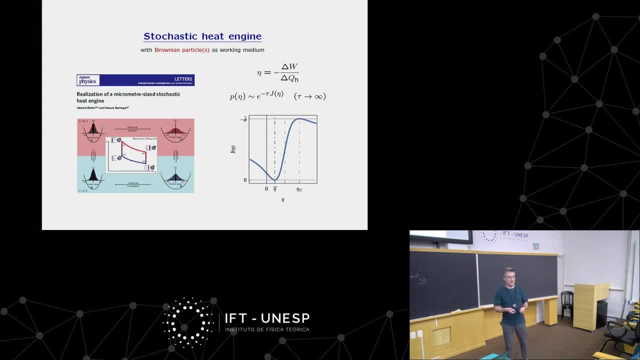 that the particle takes up, But now again it's a stochastic quantity. because these things here are stochastic quantities, They are subject to thermal fluctuations, So you don't get just one efficiency. If you repeat this experiment many, many times, you will get different efficiencies. 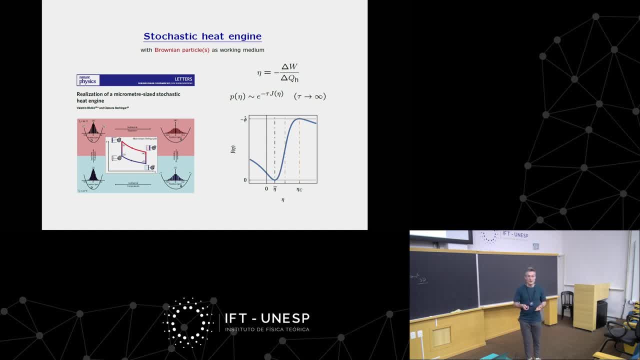 You will get a distribution of efficiencies, And now there's a very interesting result about the large time distribution of these efficiencies, If you like, in a large deviation sense. if you do this experiment for a long time, so you run this machine for a long time. 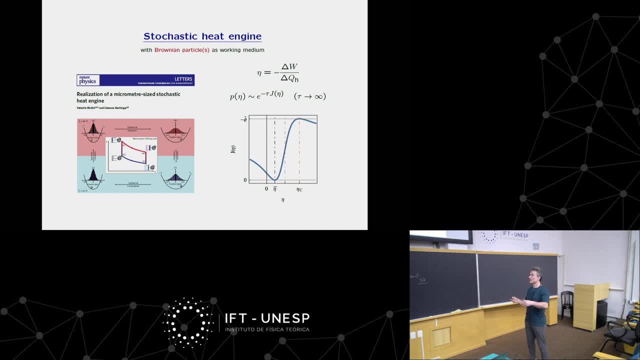 and then you repeat this machine cycling here for another long time and you look at the large deviations of the distribution- efficiency, distribution- you will find a curve like this Universally. It doesn't matter what the details are. The properties of these curves that have been shown. 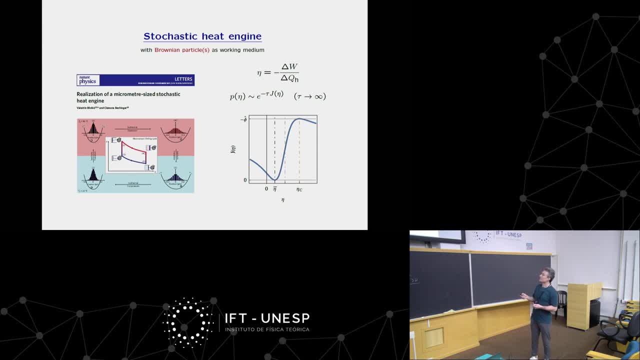 in a paper. I forgot to put the reference, unfortunately- are universal and are a consequence directly of the fluctuation theory. What does this curve tell you? The most important features are the following: This here is the minimum That means because of the minus here. 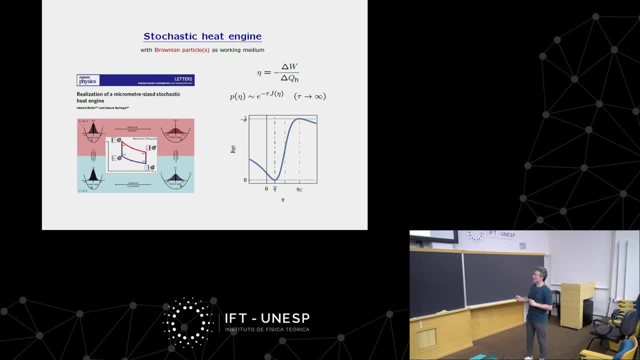 the probability of observing this efficiency is maximal. and this is the maximal. this is the macroscopic efficiency. This eta bar is the efficiency if you average delta W and delta Q. This is the efficiency that a macroscopic machine of this type would have. 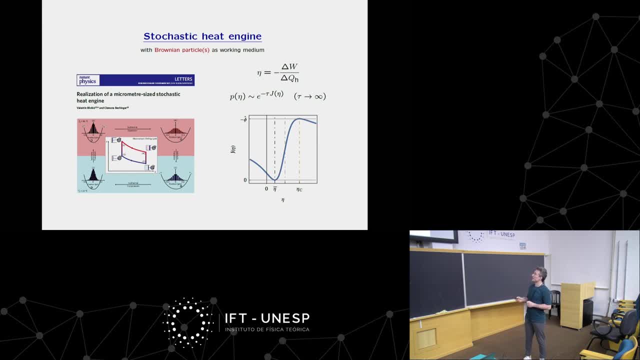 or the machine for T going to infinity. And then the other thing is that this J, here this large deviation function, has a maximum at eta C and this is the Carnot efficiency you would get for this machine. so one minus the ratio of these temperatures. 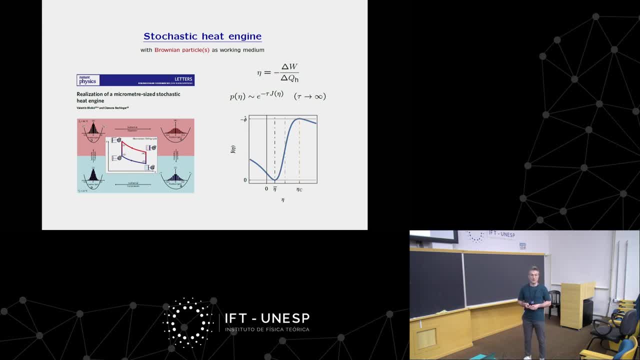 And that this J is the maximum here, tells you that the Carnot efficiency is the least likely one in this process. Okay, And this is a direct consequence of the fluctuation theorem, You don't need anything else almost. There are some technical details. 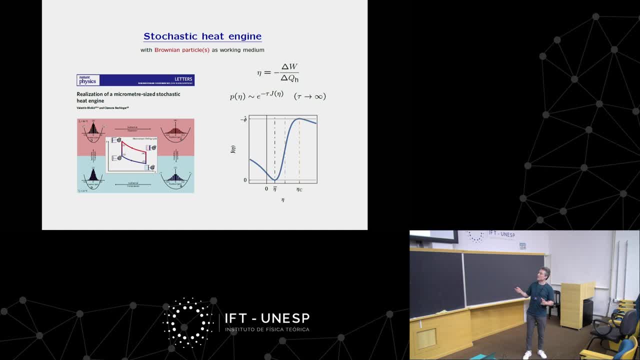 but basically the fluctuation theorem tells you that the Carnot efficiency is the least likely efficiency in such a process. Yeah, that's not an easy thing to do, So I don't know the experimental details, but they have some heating device. 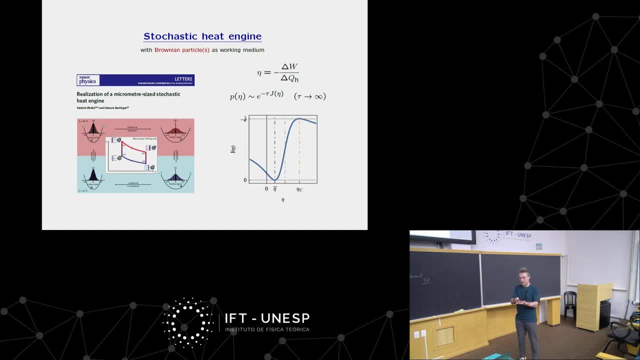 so you have to make sure that the timescales fit. So you have to make sure that the heating and cooling goes sufficiently fast so that you don't have any gradients which are interfering with your measurements. Yes, Yeah, this is related to the problem of the Maxwell demon. 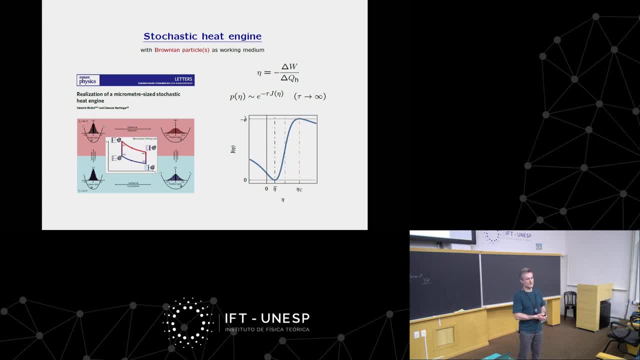 Yes, yes, and where the information loss Exactly goes. and again, there are experiments that can do that and could do such. Yeah, yeah, Exactly, it's related to the Maxwell demon. So that's one of my comments. 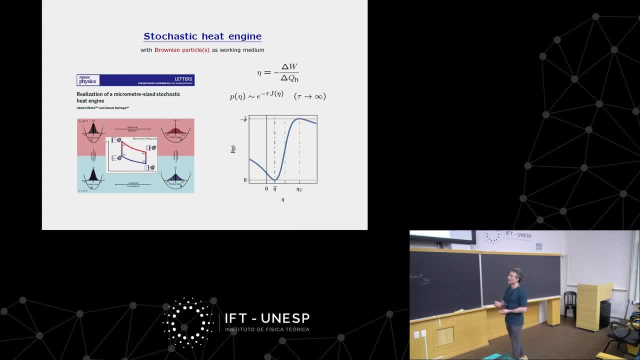 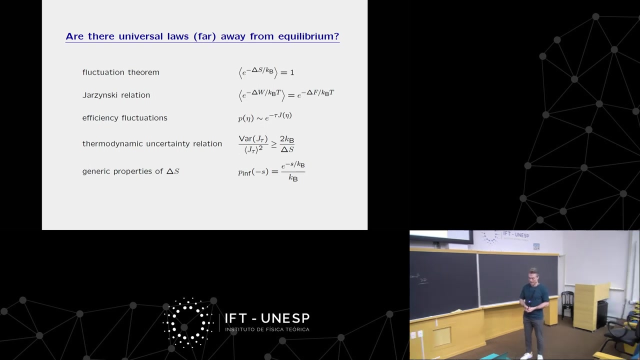 one of my prospective comments in the end, that you can actually, in this framework, include the role of information relatively easily, And information is what the Maxwell demon has to do its job. yeah, Okay, Yes. and then There's something that I find quite interesting. 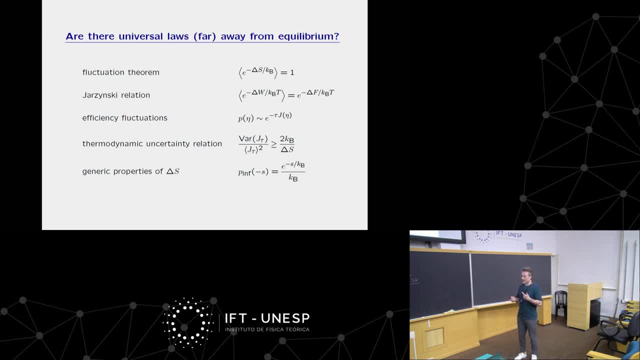 I Yeah, I gave you a framework based on the Lausanne equation, So to do these things I had to take a specific model or a model class. It's different from equilibrium statistical physics, where, in principle, we calculate partition function. 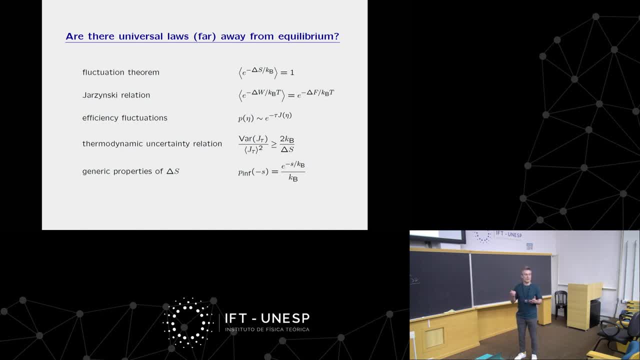 and then we know everything Here: we have to use a model and we have to use, We have to define entropy, production and work and so on, quite model-specific to get these things. But still, what I've shown to you has been done for quite different models, model classes. 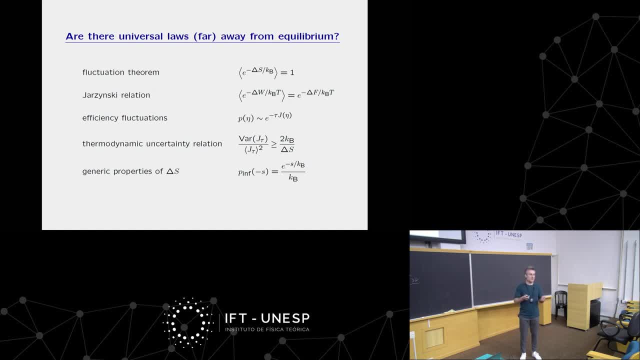 like Lausanne, equation, reaction networks, master equations, many different, And always you get these kind of results. You get the fluctuation theorem, you get the Shashinsky relation, you get efficiency fluctuations. other thing, other results. I did not explain in detail. 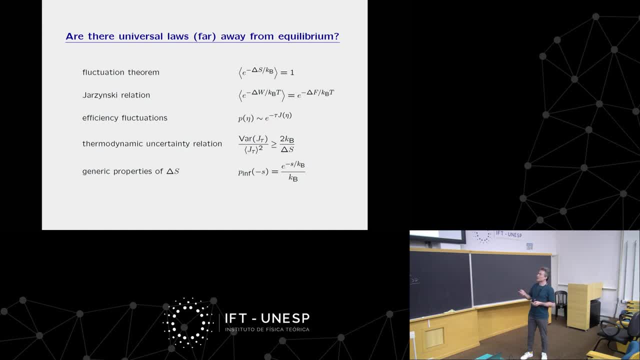 which is now called thermodynamic uncertainty relation, which gives a bound for the variations of any currents through the system. J. here is a current compared to its average, which is given by the entropy production in the system. So this is also quite universal. 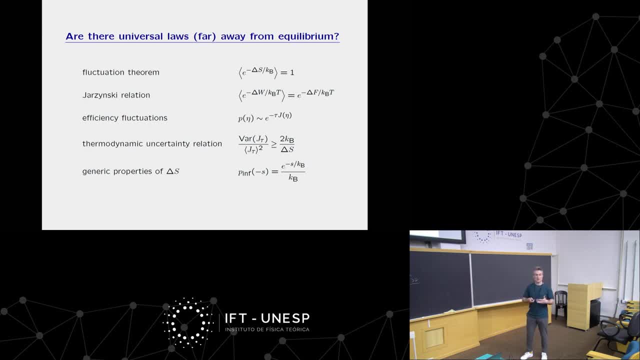 And then you also get generic properties on the statistics of entropy production. So just one more question: These relationships that you're showing, they are even stronger than your presentation, because even if I have memory on my desk, it's satisfied, right. 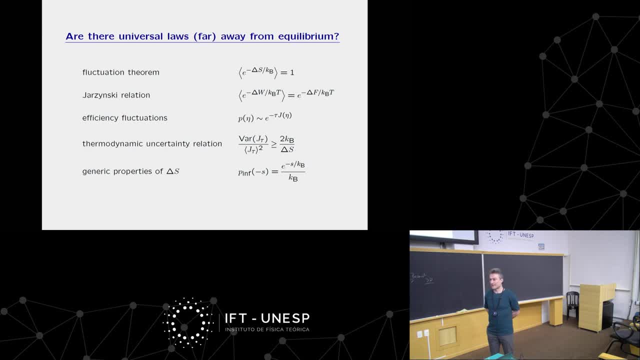 You present on a memory-free desk. It's just a Langevin equation. So the Shashinsky equation: if you talk to Chris, he's going to tell you this is going to be better. no matter what, You don't have to have a. 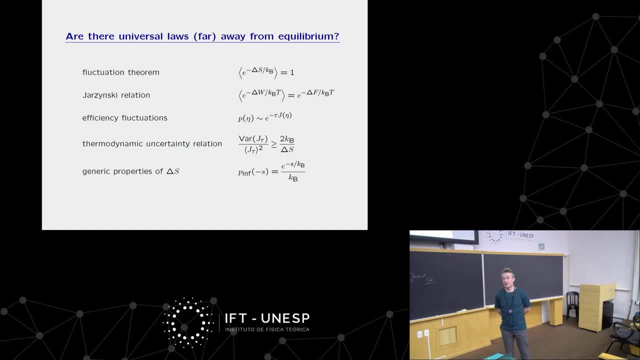 No, you don't have to have a Langevin, That's right. Right, you can have a memory kernel. Yeah, yeah, yeah, yeah, right. As I said, it's valid more generally than I present here. That's completely right. 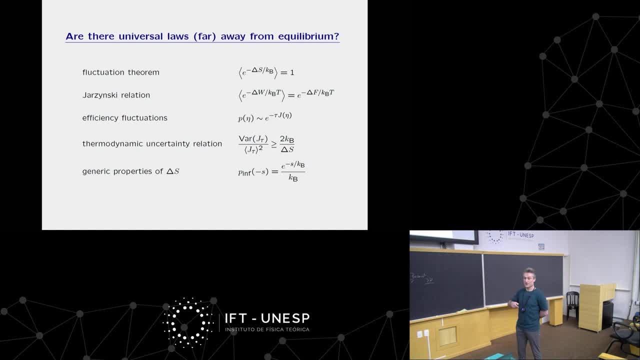 That's what I say here. There are other model classes where you still find the same relations. Okay, I'm actually coming back. No, maybe not, Let's see. And yeah, what I want to say here also the generic properties of entropy production. 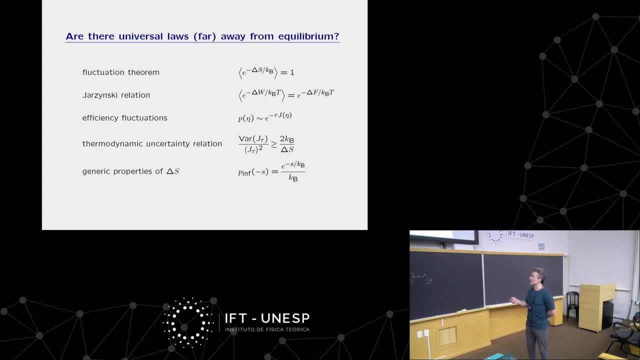 if you look at the statistics, you'll find generic properties here. It's just an example of what people derived that the global lowest value of entropy production, the minimum or infimum you get. it's also following a universal distribution which is given by that. 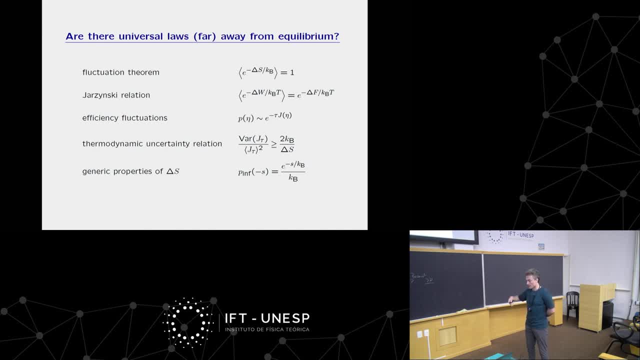 So the S here is a minus S because it's a negative value. the global minimum, The statistics of that it follows, also universal. So there are these things which pop up every time you understand how you have to do thermodynamics with models which are, in principle, 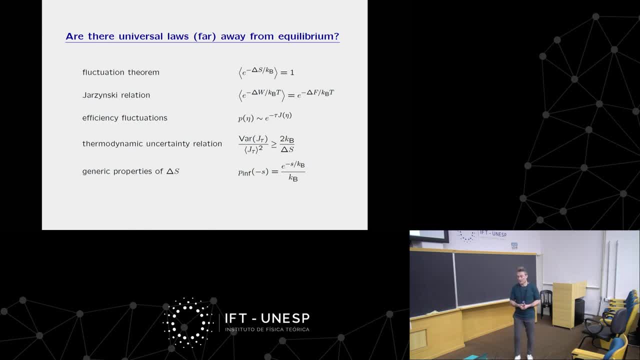 describing dynamics of systems, small systems where fluctuations play a dominant role. And the question is then: are there universal laws, even in non-equilibrium? Is there? I mean, this is the dream almost from the very beginning of the development of statistical physics. 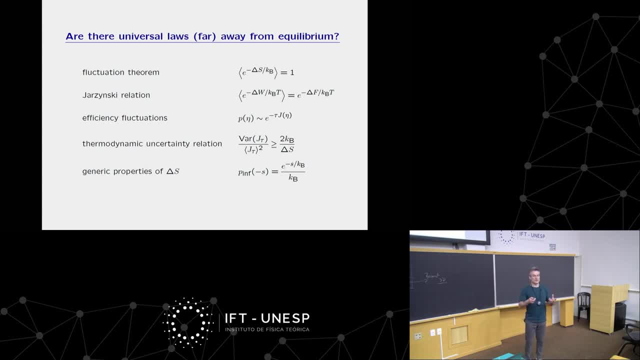 that you can find universal laws also in non-equilibrium situations, not only equilibrium, And people are often saying these laws are valid far, far from equilibrium, which is related to the fact that you can do whatever you like with this protocol. You can drive the system very well. 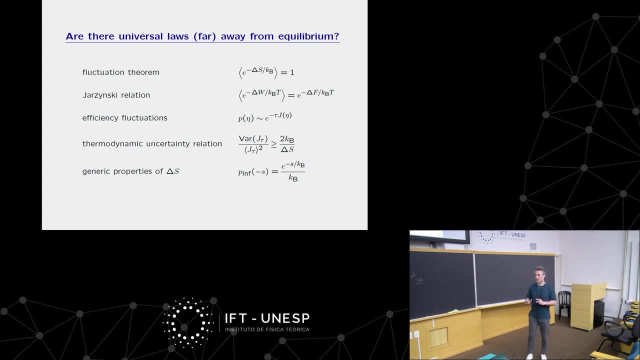 and very fast. But I would like to add: there is one restriction And here is one basic assumption always, namely that the path your system is connected to, the path which it can exchange heat is in equilibrium. So, no matter what you do, 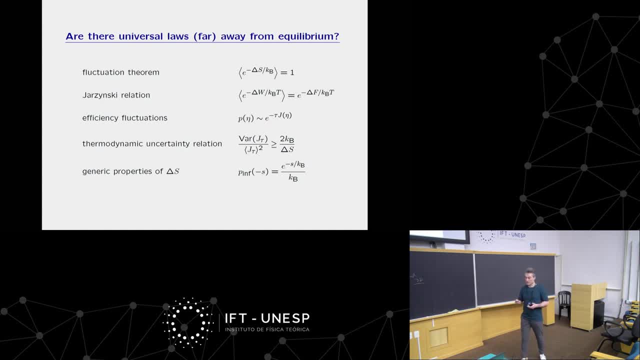 the path is always in equilibrium system And this of course also limits somehow the timescale. If you're driving your system so fast that you're reaching the characteristic timescale of your path, then these things, I would say, break down. 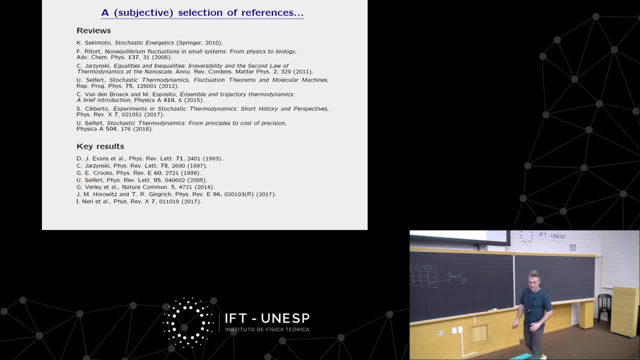 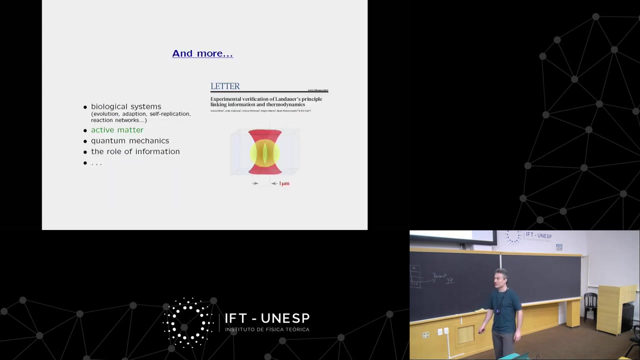 Okay, Here is a subjective selection of references, a few reviews, and here are a few key results. Some of them I have presented here, some not. I will show this slide again, so you don't need to take photos or copy. I would like to go to the perspective part. 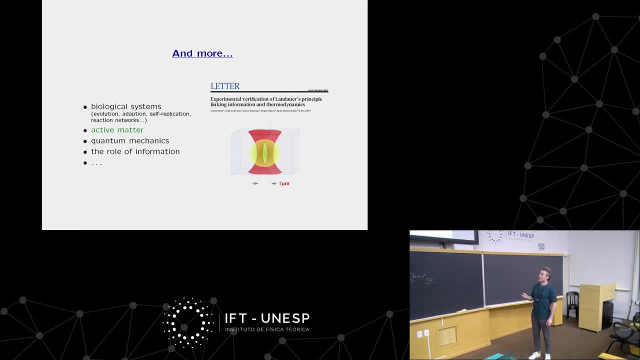 a little bit in the last 10 minutes So there is more. So I presented for Lausanne equations, But more generally you can apply these concepts or develop these concepts. I should say for biological systems There are attempts in evolution. 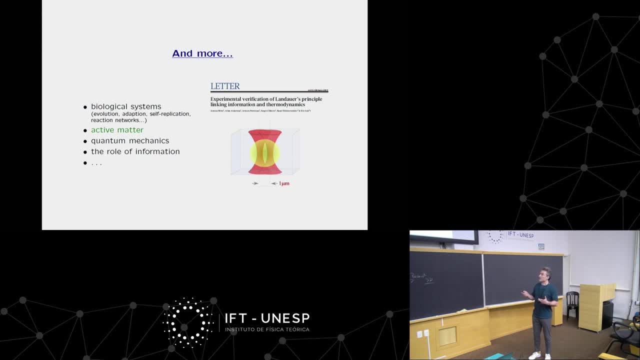 adaption, self-replication, reaction networks- a little bit related also to what Marco presented this morning. And then there are attempts now to develop these kind of tools for active matter, And this is also something I'm personally interested in. so I can say a little bit more after that slide. 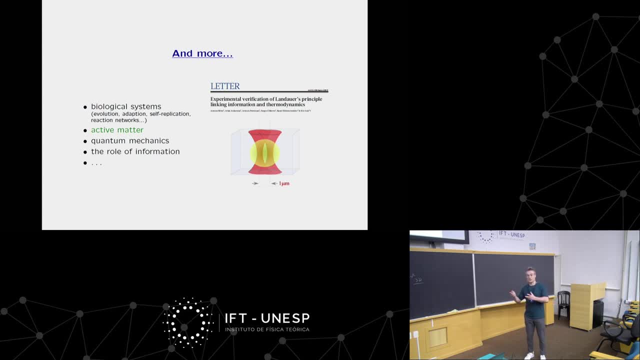 Then of course, quantum mechanics. I also only presented classical model, Same ideas. What can you do with quantum mechanical systems? And then the role of information. It can quite easily incorporate it here. And there's another example for a very interesting experiment. 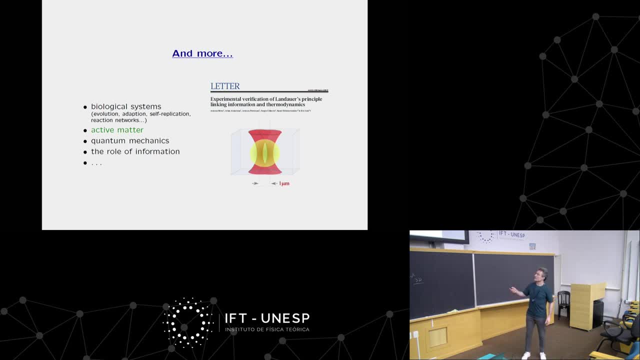 People did again with colloidal particles and optical tweezers. This here is representing two optical tweezers, So this creates a double-well potential for a colloidal particle. And this is like a bit of information. Left hand is one, right hand is zero, maybe. 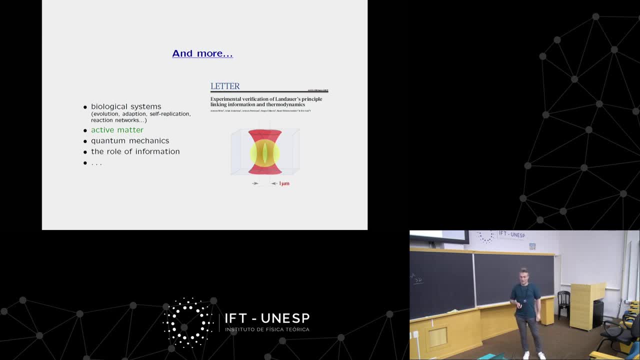 And then you can measure the entropy it costs to erase a bit of information or store a bit of information, And you find Landauer's principle, where the upper limit is Kb ln 2. So you can do these things, And then you can also develop a theory. 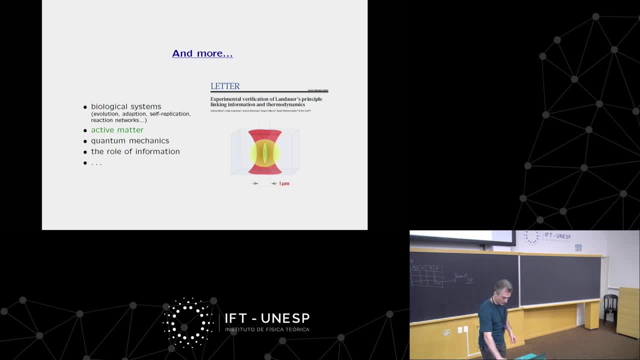 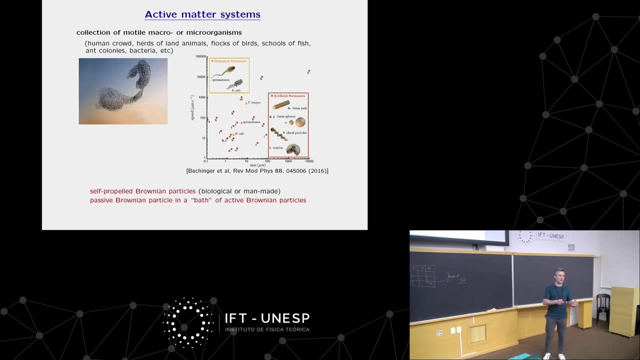 incorporating information in that framework. So a few short words about active matter systems, Also because they are part of our school. Julia is going to talk about active matter systems And these systems are a collection of motile macro or microorganisms, So like human crowd. 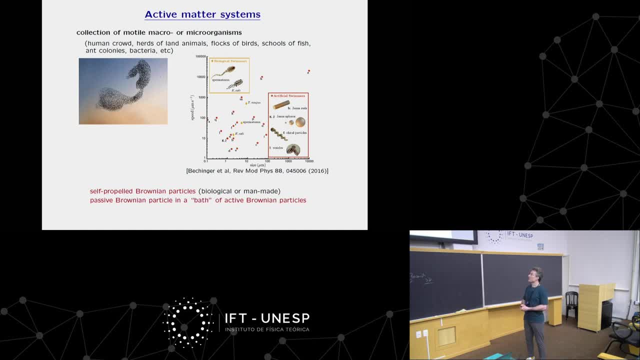 herds of landowners, flocks of birds, schools of fish, ant colonies, bacteria and so on. And when I talk about active matter systems coming from this colloidal particle perspective, I always have in mind a self-propelled Brownian particle. 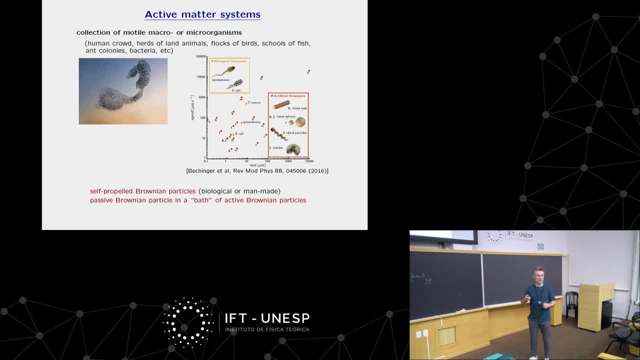 So basically a Brownian particle which can move on its own. You can say a bacteria is a Brownian particle which can move on its own. So systems like that I have in mind. There are still thermal fluctuations which play a dominant role, but the thing can self-propel. 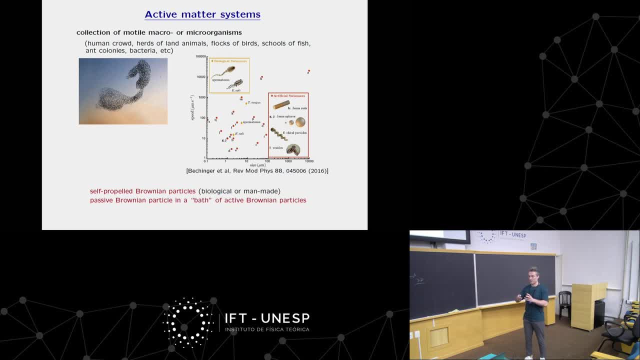 move on its own, Or it can even be a passive Brownian particle, a passive tracer, which is suspended in a bath of bacteria. So this tracer particle is then not only pushed around by the water molecules, but it's also pushed around by the bacteria. 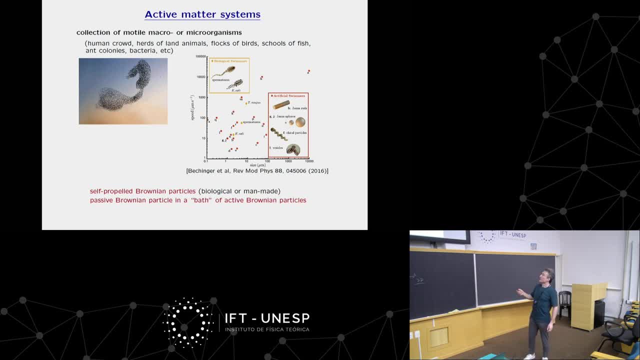 moving actively through the solution, And here it's taken from a rear view. This is a plot plotting this kind of self-propelled Brownian particles up to a millimeter in size. speed versus size, Just to see. there are biological and artificial swimmers here listed. 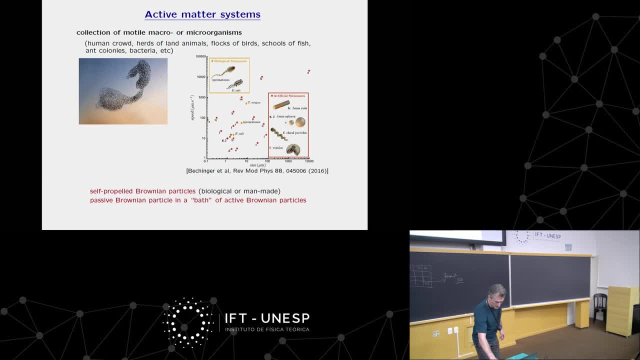 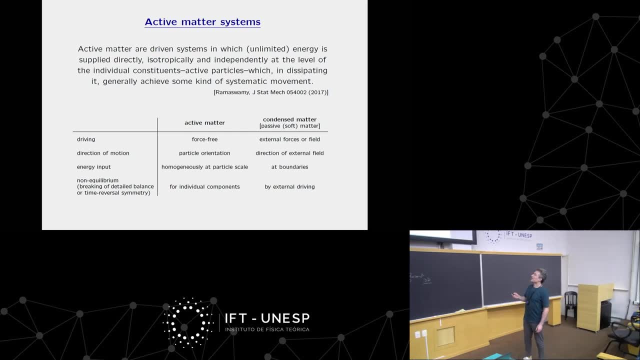 So people do a lot of experiments with these things right now, And if you look for a more detailed definition of active matter, I found this one in another review. Active matter are driven systems in which unlimited energy is supplied directly, isotopically and independently. 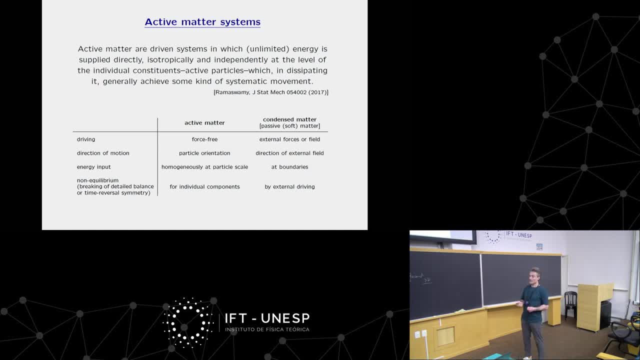 at the level of the individual constituents, the active particles which, in dissipating it, generally achieve some kind of systematic movement. So you're not in this description, you're not concerned about where does this energy supply come from. They just have it, they convert it. 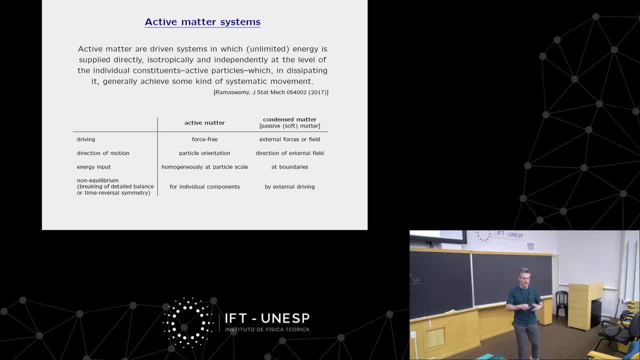 and they move. And this makes these systems generic out-of-equilibrium systems, which are different from the out-of-equilibrium systems I described before, Because the passive particle: if you want to drive it out of equilibrium, you need to apply force. 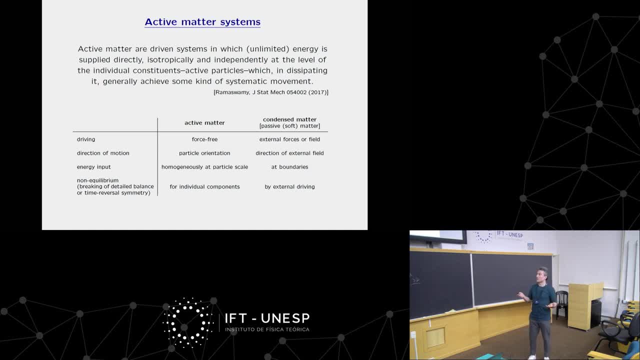 Here these objects move on themselves, so you don't even need to apply force. This is a comparison here. the table, The classical condense or passive soft matter particles, they, if you want to drive them, the external forces or fields. 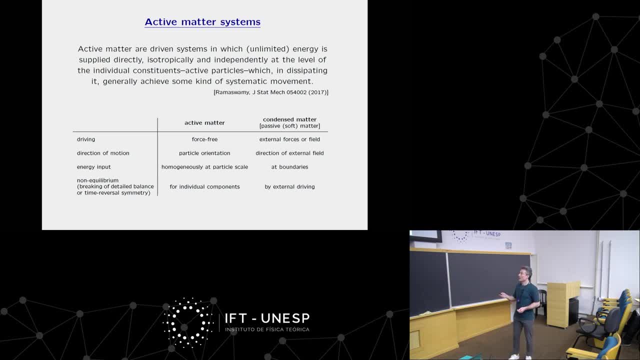 and here the driving is force-free. They move on their own if you like, And the direction of motion is usually connected to the orientation of the particles, so it moves over time diffusively. very often Here it's given by the direction of the external fields. 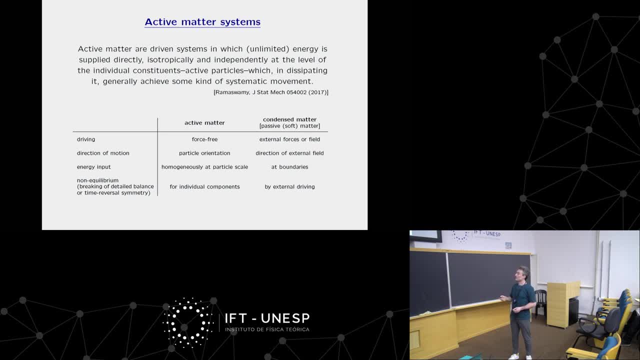 Energy input, as stated in the definition, is homogeneously at particle scale. so you feed in energy into the system on very small scales and this gives rise to some new unexpected effects, And here the energy is supplied at the boundaries. 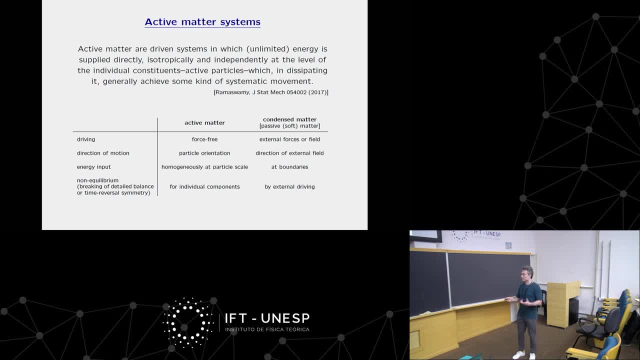 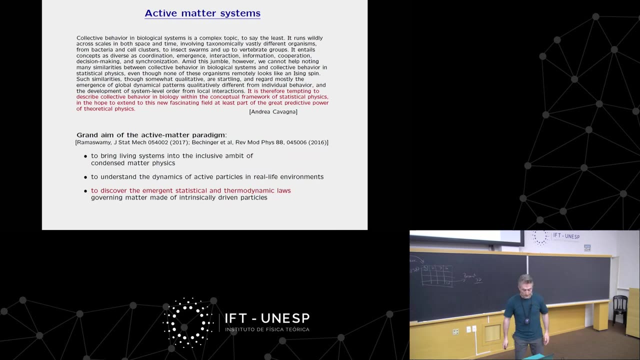 if you like. And then non-equilibrium, breaking off detailed balance. here this happens for individual components and here you have to apply an external driving to do it. So there are quite some differences, but still, if you observe these systems, 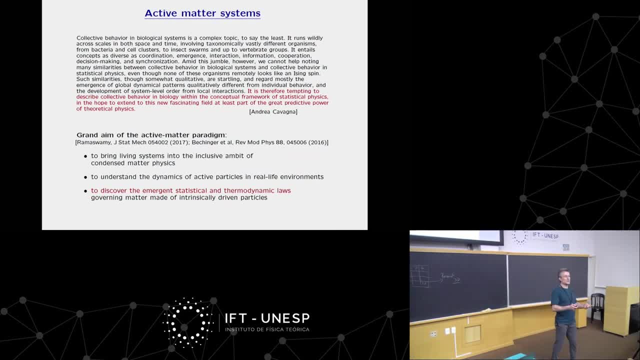 very often they look like what we are used to from statistical physics. They have very similar properties and the best description of this I've seen so far is from Andrea Cavagna, from Rome, and he wrote- I think it was an abstract of his talk at some meeting I was: 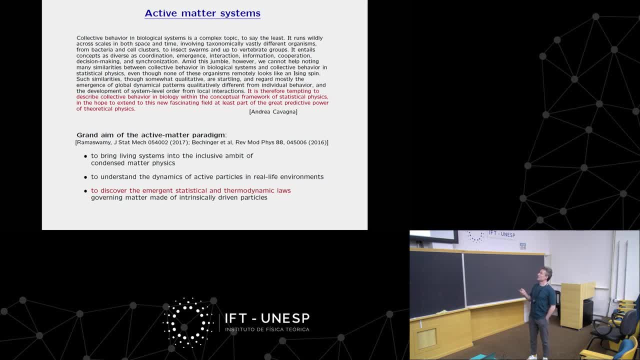 So the collective behavior in biological systems is a complex topic, to say the least. It runs widely across scales, microorganisms or herds of animals in both space and time, involving taxonomically vastly different organisms from bacteria and cell clusters. 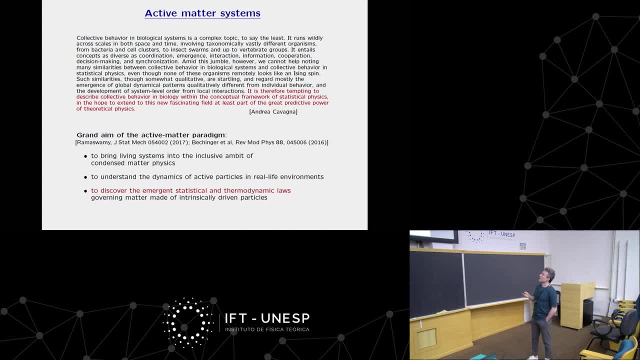 to insect swarms and up to vertebrate groups. It entails concepts as diverse as coordination, emergence, interaction, information, cooperation, decision-making and synchronization. Amid these jumble, however, we cannot help noting many similarities between collective behavior in biological systems. 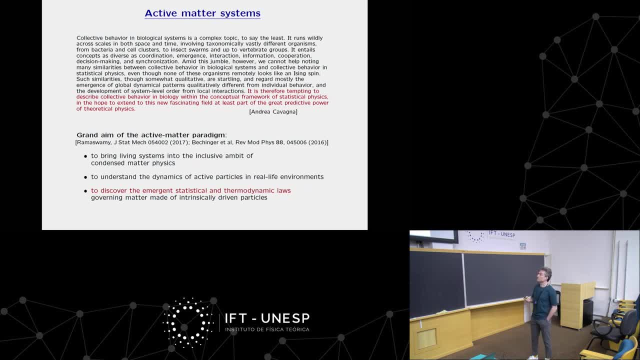 and collective behavior in statistical physics, Even though none of these organisms remotely looks like an icing spin. Such similarities, though somewhat qualitative, are startling and regard mostly the emergence of global dynamical patterns qualitatively different from individual behavior, and the development of system-level order. 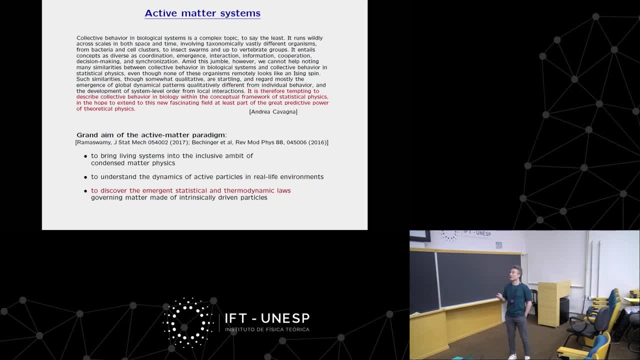 from local interactions. This sounds very familiar, right. It is therefore tempting to describe collective behavior in biology within the conceptual framework of statistical physics, in the hope to extend to this new fascinating feat at least part of the great predictive power of theoretical physics. 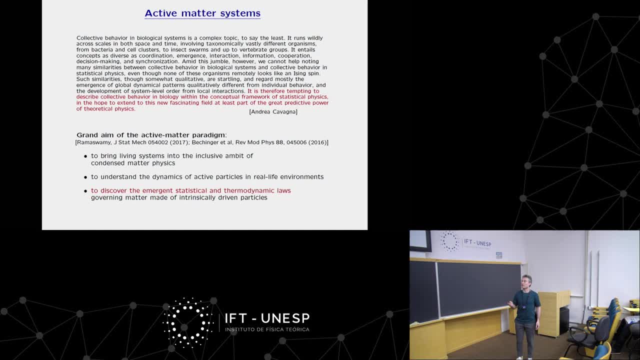 So this is actually the whole idea behind active matter, And other people say the grand aim of the active matter paradigm is to bring living systems into the inclusive ambit of condensed metaphysics, to understand the dynamics of active particles in real-life environment, and here 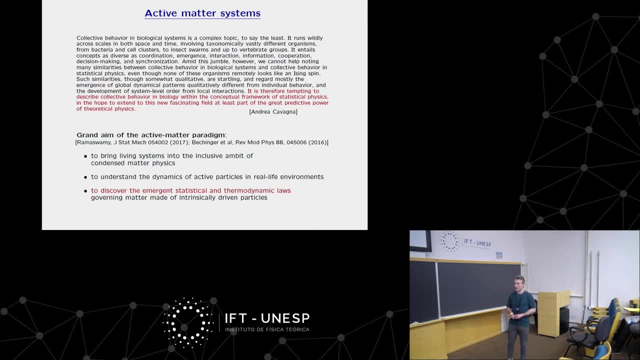 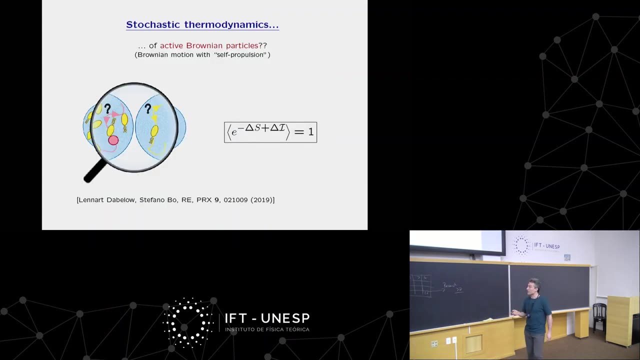 to discover the emergent statistical and thermodynamic laws governing matter made of intrinsically driven particles. And this is the part where I'm interested in a little bit and I try to approach this from a stochastic thermodynamics perspective. And just very briefly, 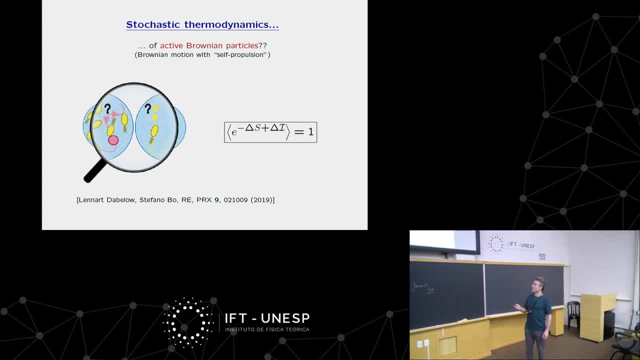 so these are the systems- either bacteria that move in solution, active particles themselves or a passive brownian particle pushed around by bacteria- And we tried to develop a similar approach as for stochastic thermodynamics, asking about the irreversibility, comparing probabilities for observing. 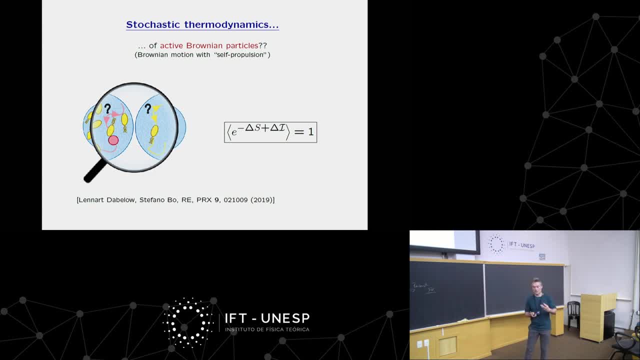 certain trajectories forward in time and backward in time, Because this question, as we learned from the passive case, is connected to the entropy production. So to the question: what is entropy in such a system? This is much less clear for active particles. 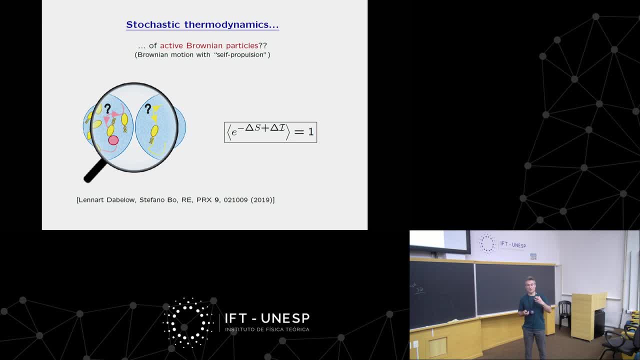 because it's an out-of-equilibrium system per se And there is actually quite some confusion. There are at least a handful of different suggestions of how to define entropy production for these kind of systems. What we found with our approach for a brownian particle. 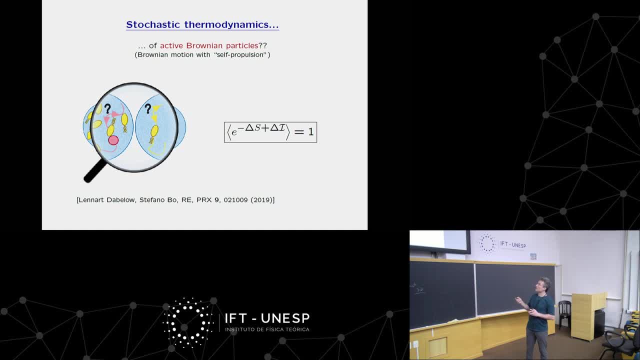 with self-propulsion is that you get a fluctuation relation which very much looks like the one I've shown you before, where here is the entropy production of the entropy production in the bath, which is connected to a certain trajectory, but then you have another contribution. 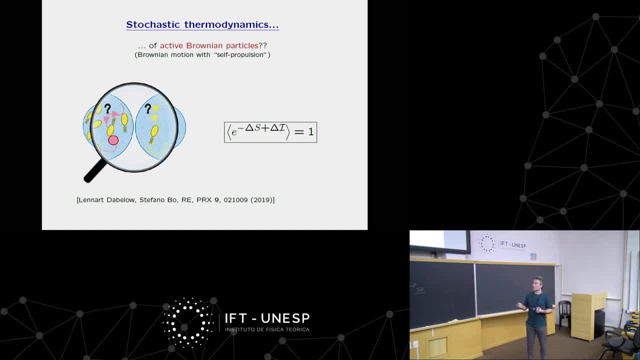 which is related to the correlations that this trajectory has, let's say the trajectory of the passive brownian particle here, the correlations it has with the movement of the bacteria, which are out-of-equilibrium, so that you cannot define an entropy. 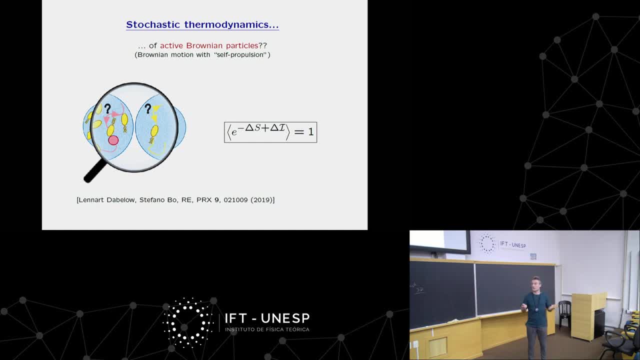 for the bacteria bath. It's a concept that doesn't make sense. So this contribution here from the bacteria can be ascribed to what we found by the correlations which are here written in form of an information theoretic concept, which is called the mutual information. 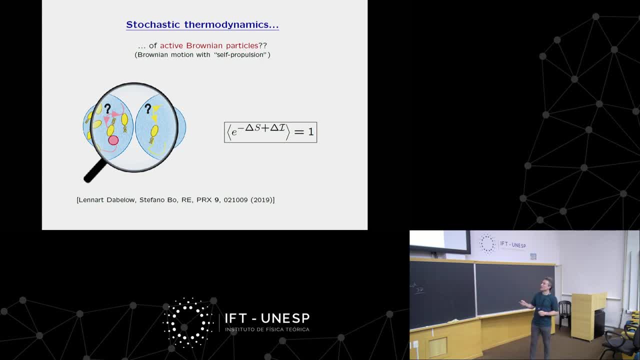 I don't want to say more. This is just what we found: that you can derive fluctuation theorems but you get a different contribution. So you can also see coming back to the role of information if you want to interpret it in a different way. 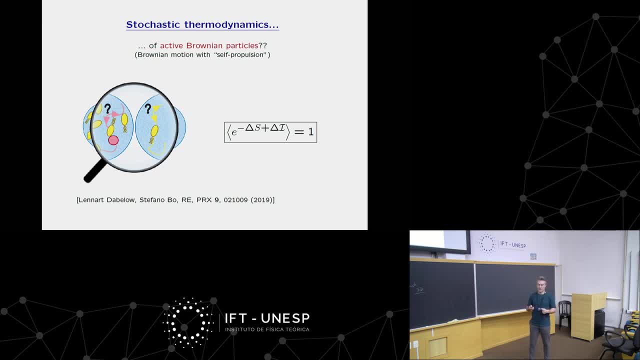 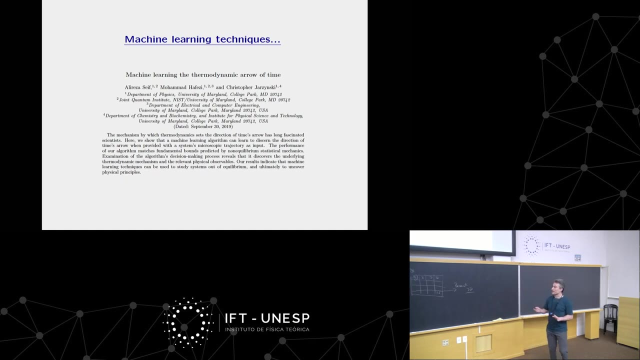 you could say that these things provide the reservoir of information. Okay, Which contributes to this fluctuation theory. Okay, And another thing that very recently popped up. I must admit I didn't read this paper yet, but I wanted to show you. 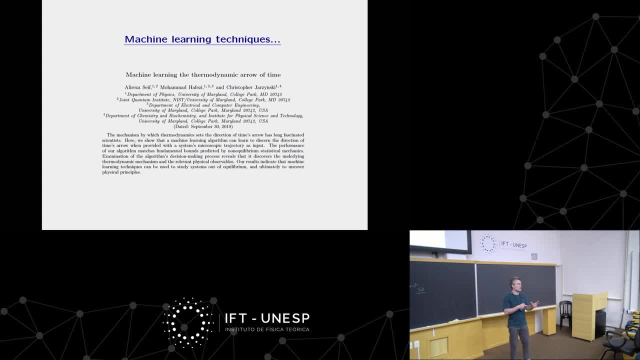 because I found it recently and because also at this school we have a lecture actually on neural networks and machine learning, that people start to apply machine learning techniques to these kind of systems. And this is Chris Szczesinski- again the guy from the Szczesinski School. 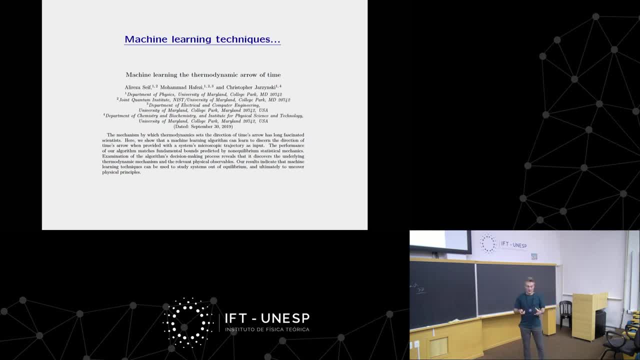 he's a professor at the University of Chicago and he's a professor at the University of Chicago and he's going to talk about the relationship between the machine learning and the machine learning. And what they did: they tried to estimate the error of time. 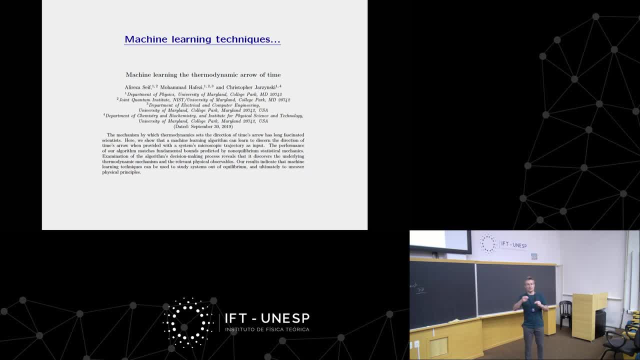 or determine the error of time by exactly what I described before: by letting the machine learn to distinguish between movies played forward and backward in time. So you present microscopic trajectories forward in time and backward in time. let the neural network learn and let the machine learn. 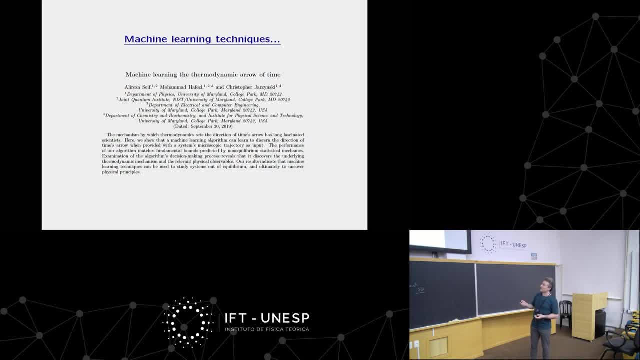 to distinguish between movies played forward and backward in time, And what they found is that it seems to work very well. And more interestingly, I think that they say: the performance of our algorithm matches fundamental bounds predicted by non-equilibrium statistical mechanics. Examination of the algorithm's 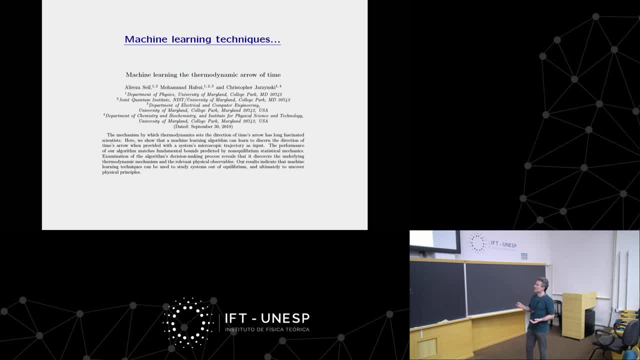 decision-making process reveals that it discovers the underlying thermodynamic mechanism and the relevant physical observables. This, I think, is quite interesting. I said I cannot say more about this paper because I haven't studied it myself in detail, but you can. 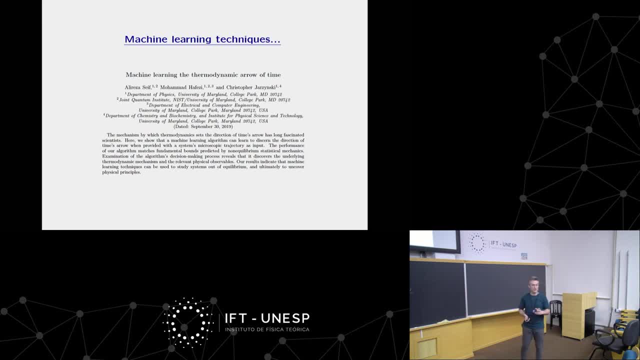 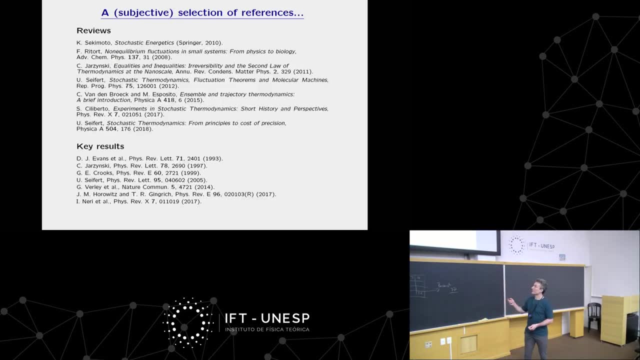 This is from archives, so you can Google the title, you will get it and you can read it yourself. And with these remarks and perspectives I'm at the end of my talk and here is again the list of the reviews I recommend to read. 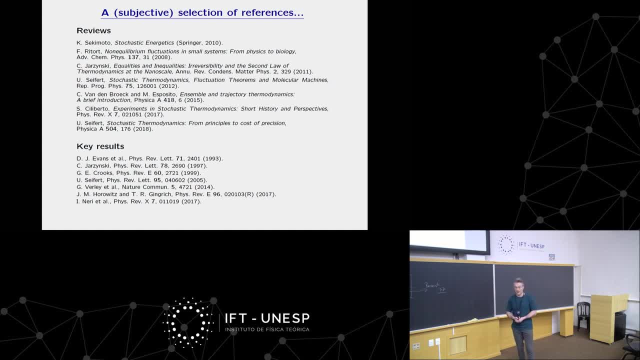 if you are interested in that topic in more detail, and the list of papers with some key results. Of course, it's a subjective selection and by no means covers all the contributions that have been made to the field. Thank you very much for your attention. 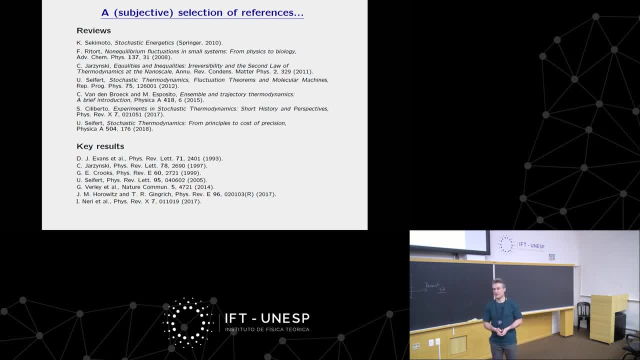 Thank you for a very nice lecture. I think it was interesting. This is all very controversial. Yeah, I know Chris for a long time, so does you, but it's an interesting question, But the question I really like in the end. 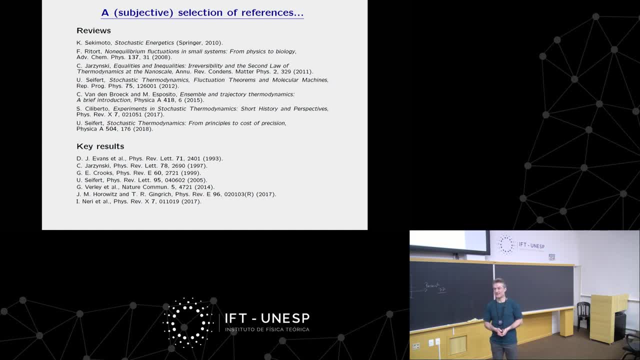 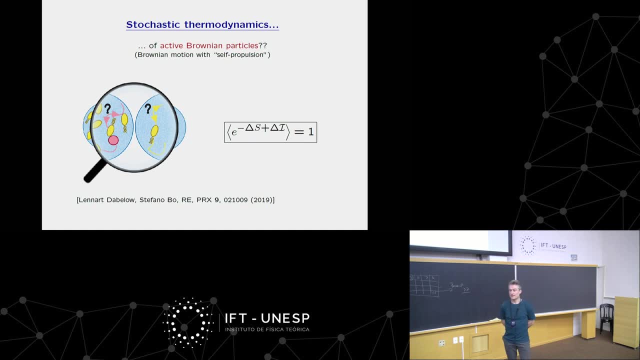 when you're talking about active materials and you're doing this model where pretty much you have like a Brannion particle plus sort of a kicking motor that can kick anytime in any direction. We like to use the word smart matter where you have an active matter. 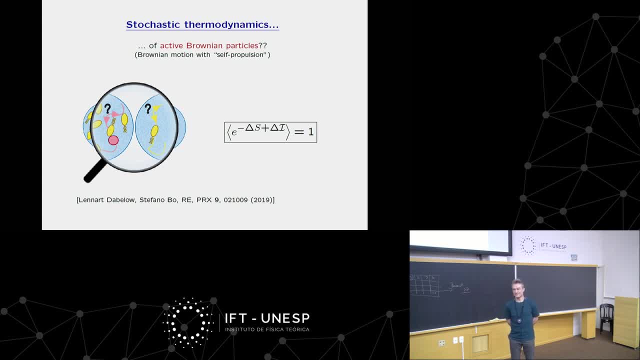 driven by information. Do you want to comment a little bit more about that? It's a word we have been using in the past that basically you think biological matter would make an interface to that. how you put information driving active matter. Information driving active matter. 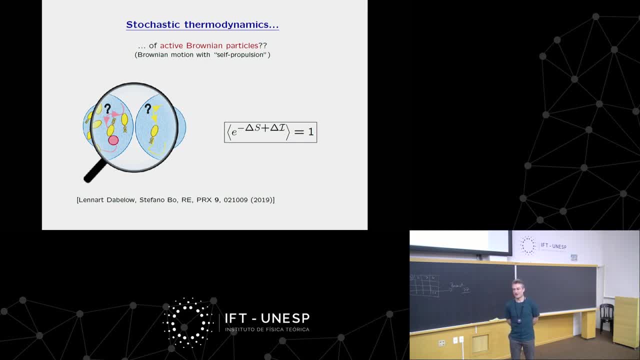 That's what happens in biology. right, These motors are kicking, but somehow you have a signal, for example, from a chemical network that pushes up a mechanical system, Chemotaxis and things like that Exactly, For example, or any process like 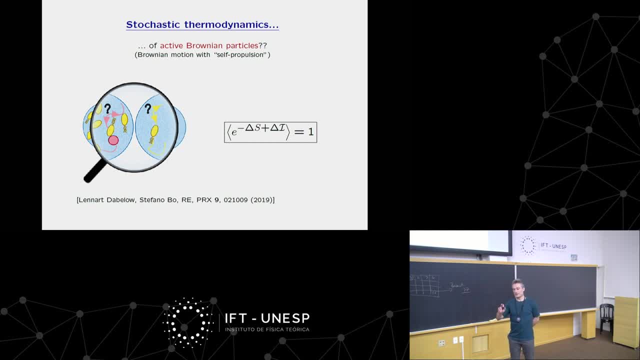 epithelial mesenchymal transition or any process in biology. you're giving information to an active matter to behave. Yes, I don't know these works so well, but I know that there are quite a number of papers which include exactly this information aspect. 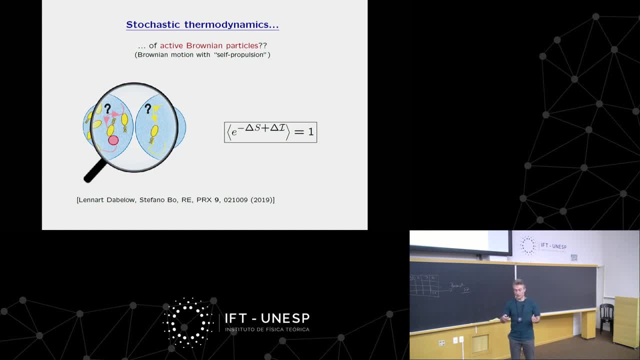 into the whole framework And then what you find with these inequalities that you get: bounds on how much information you need to perform in a certain way or to adapt, and things like that. So this framework provides instead of: I mean, the second law is a bound right. 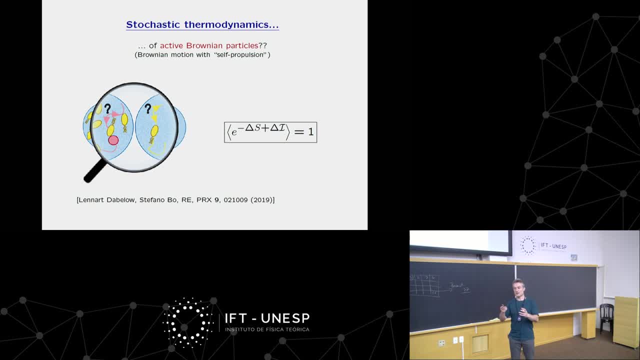 For the entropy production, And in these cases you get bounds for adaptivity or for performance or speed versus adaption and things like that. Right? I get very interested in all the timescales. right? You just told about the Jarzynski inequality. 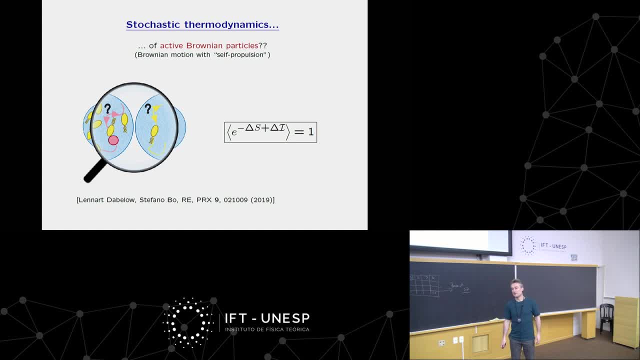 So it's always true. but if you push your system too fast then you're going to need like a very large number of trajectories on that average to have any chance of getting a result right. So in a sense it's sort of a. 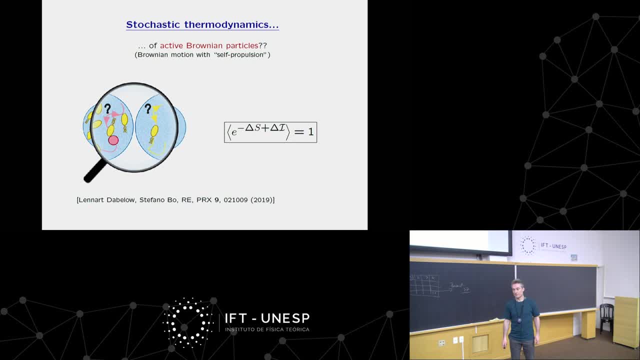 No, this is. That's why the Pustamante is so important. I mean, the Pustamante is so important because it allows: the experiment that you present is far from being a total agreement among people, You have letters and letters. 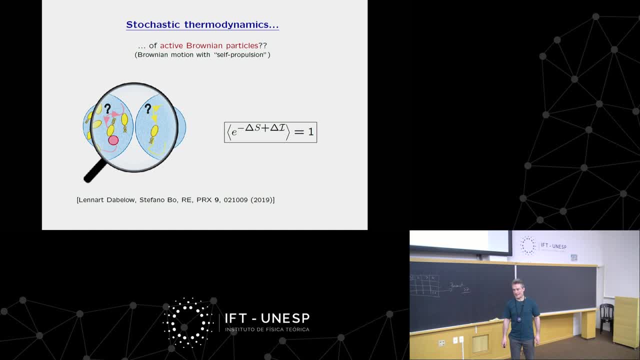 So in a sense, the question of timescale. you raised the question just about the bath, that if you go so fast that the bath cannot Follow, yeah, Follow, it becomes a problem. But even there, But for an equal solution. 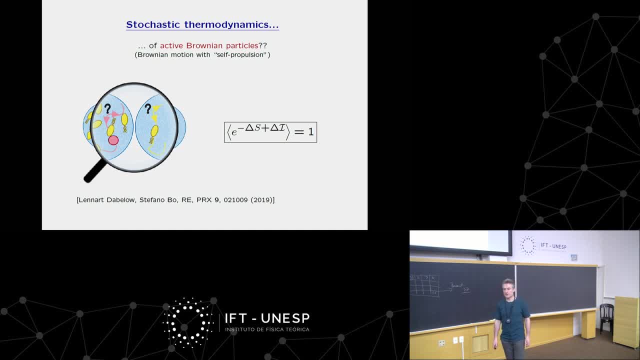 this timescale is, I think, 10 to minus 13 seconds or something like that, So it would be difficult to do an experiment on the timescale. I understand, No, no, But if you use the Jarzynski equation, 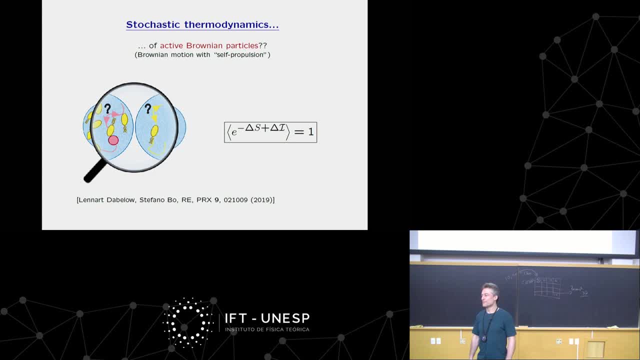 for example, people that do simulations. they do a simulation very fast and they try to compare it with experiments on a much longer timescale. right, That's what used to do that a long time. Lots of people used it. Then you may notice. 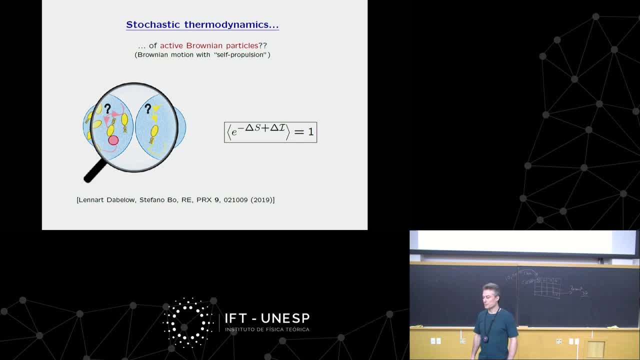 that you may need a very large number of trajectories to. actually, I think this problem is more related to the fact that, in this average, the tails have quite a large contribution. Exactly, And to get the tails you need a lot of Right. 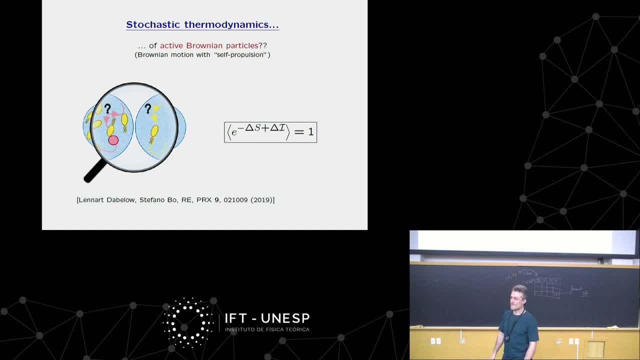 And the faster you go, the more you become tail dependent. Oh, you don't need the tail, right, Exactly, exactly, Yeah, okay, But I think it was very nice. In that sense, we agree. yeah, So can you give? 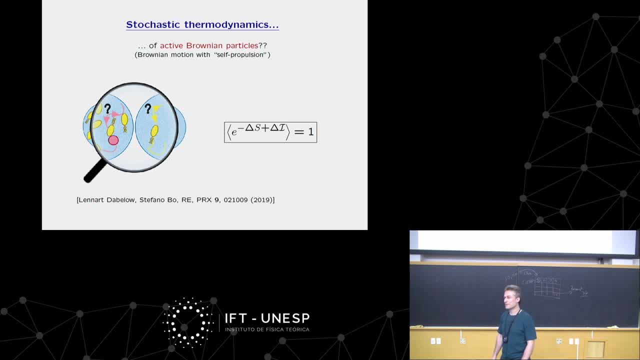 an explanation of exactly how does this feature in biology works, for example in self-reproduction. How can the Langevin equation model this phenomenon? No, it's not using the Langevin equation. In that case, people use more like these reaction networks. 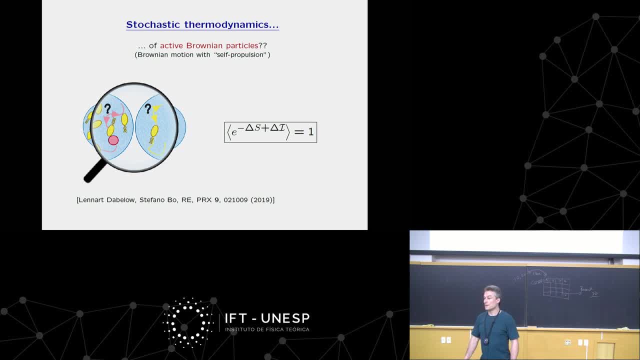 and then master equations, And then you can also for this class of models- I have not presented them at all- You can also write down entropy, production and heat and so on and so forth and develop a similar formalism. Okay, And then 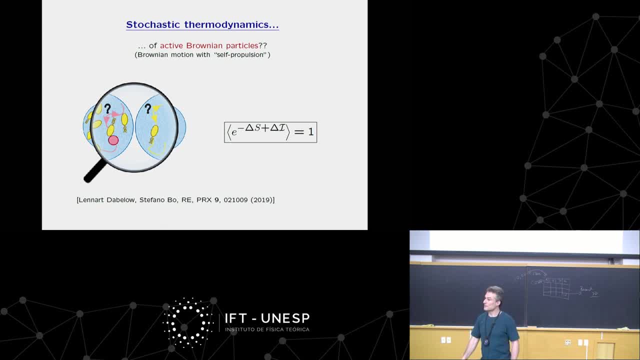 you get similar results and can derive these bounds. So it's not that in the Langevin equation you can code that the biological system self-reproduces itself in some kind of No, no, Usually no, you don't use the Langevin equation. 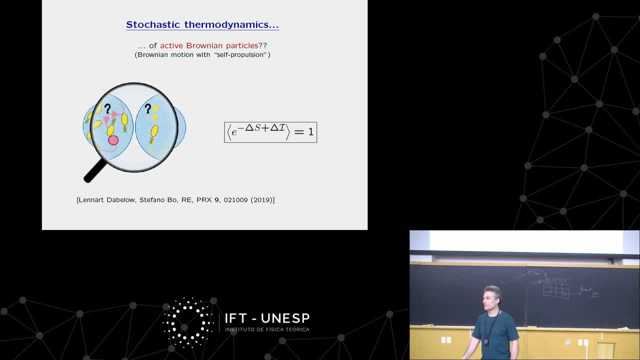 for these kind of questions. Okay, Thank you. Well, I think another smaller scale example are motor proteins, because they are driven by Brownian motion Right, And another system which would be very interesting is to study the well, what you would call. 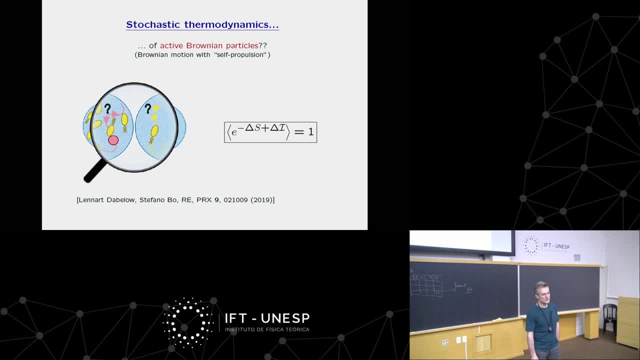 embryology, how, from an initial oversight, the whole organism developed, because there are beautiful experiments showing. following this, it is a completely self-organizing system. You have a huge number of cells and then they build up the organism spontaneously. Yeah, yeah, yeah. 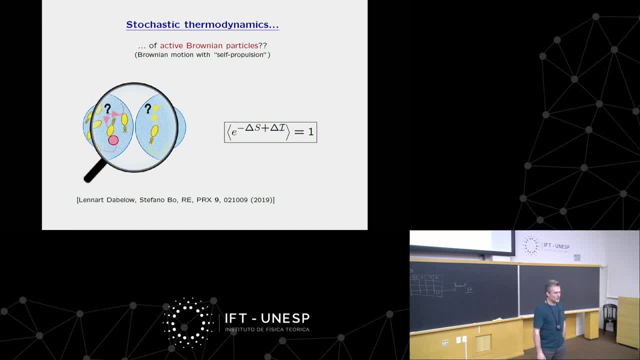 so there are also attempts within this framework to quantify the costs of self-organization, the thermodynamic costs of self-organization and so on, and give bounds and what is the dissipation, and so on. Now, that's also possible within that framework. And the heat bath: 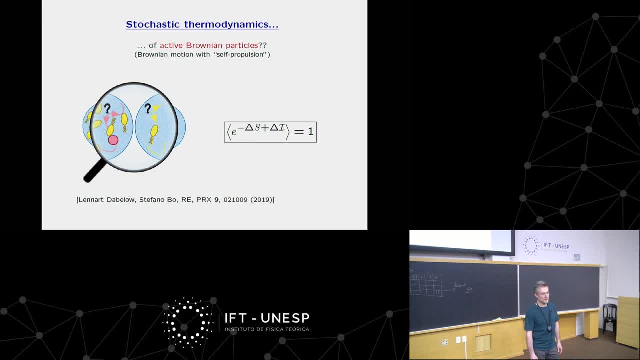 that drives everything, of course, is the sun. Yes, Hey, I have a question. So it seems to me that it's important to have, like, the overdump limit to write the stochastic thermodynamics, right? No, no, it's not. 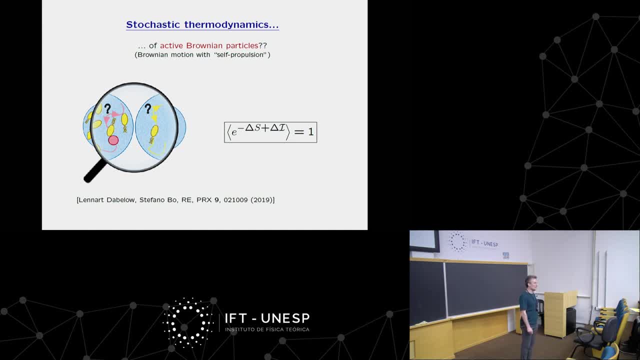 It's just for me it's not. So you can do the same thing in having the inertia term there as well. Then you simply have the kinetic energy as another contribution. The second of the derivative in time is another contribution. Yes, 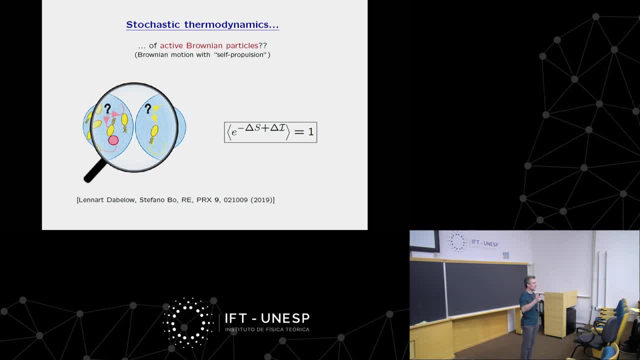 yes, it will. this will be a contribution: one half mv squared the kinetic energy, and this will contribute to the energy balance and then the motion. So this time the energy will continue to be energy of the center, of the center, of the center. 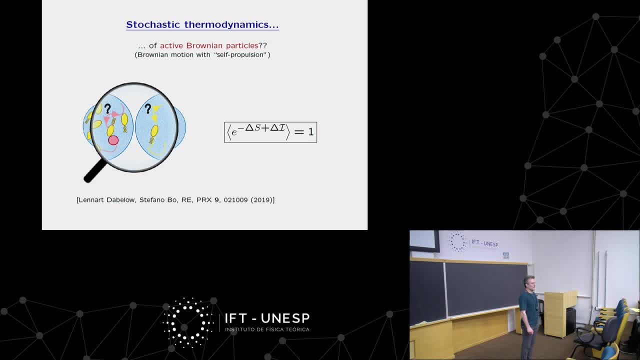 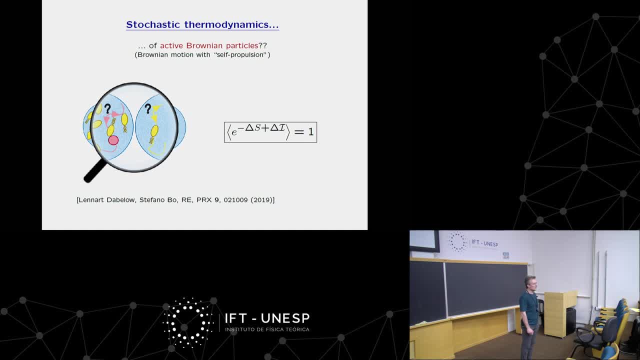 write a Langevin equation for some other parameter. right Yeah, you can do that. I guess This probability distribution came from experimental results, or I don't get where this distribution came from. Which distribution do you mean, For example, probability? 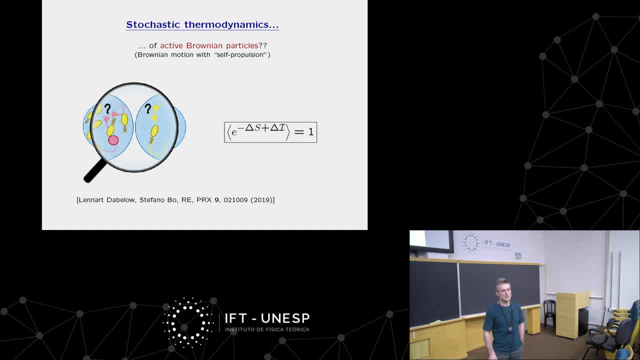 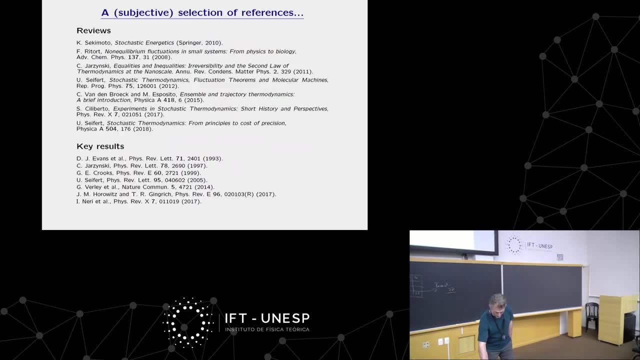 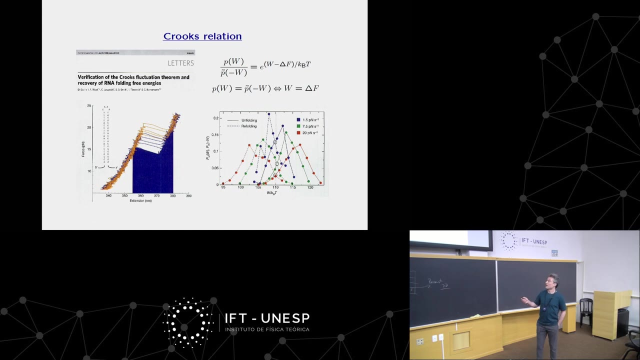 to came and to back. Okay, how can I find this distribution? Do you mean, for instance, this distribution's here? Yeah, these are from experiments. If you do the experiment with this on a hairpin, you start in a folded configuration. 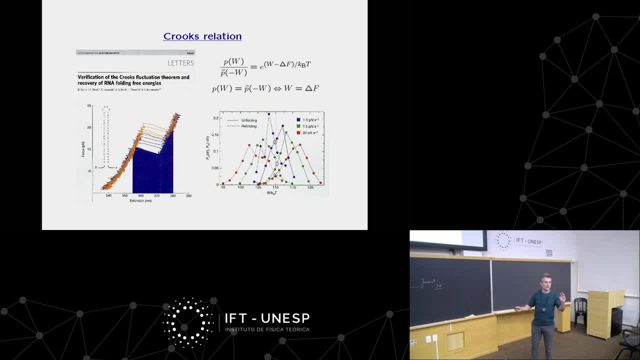 and one of the ends is somehow connected to a colloidal bead which you trap with a tweezer. so you can pull, you can apply a force at this end, say, and then at some point the whole thing unfolds. And since you can monitor, 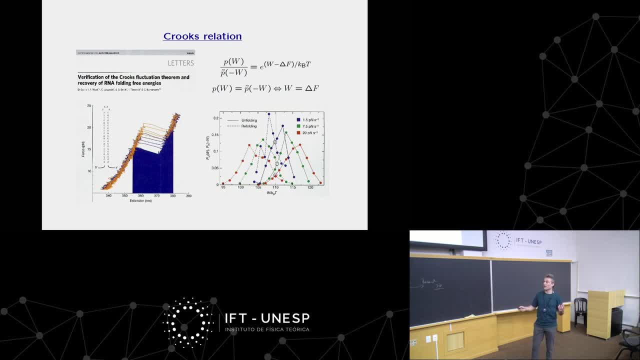 the extension and the force you're applying, you can get the work which you perform on the system during the experiment. So for one of these curves, you get a value for the work. then you let it refold, you get a value for the. 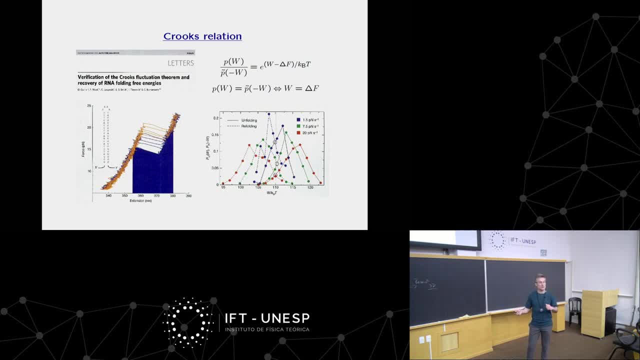 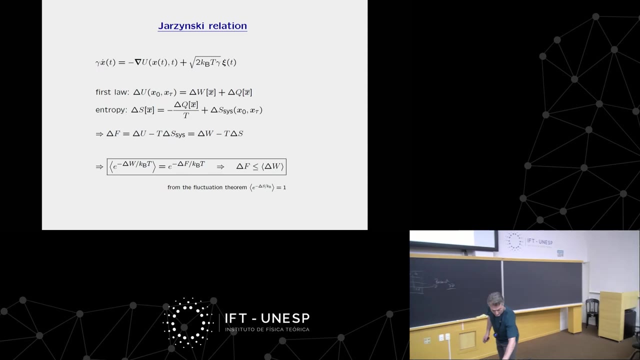 work in the reverse process and then you repeat this experiment many times and collect all the work values and from that you get a distribution. Okay, This is in the experiment here, The distribution I wrote down. let's say here, for instance: 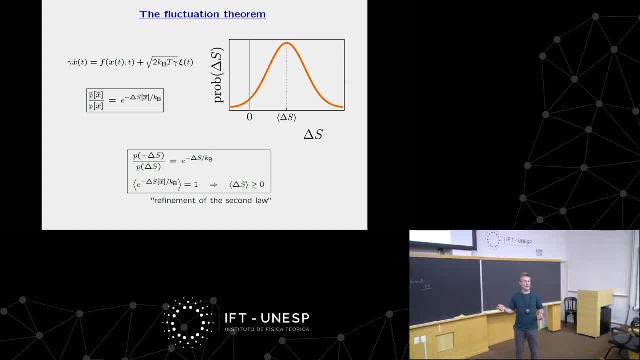 these distributions you can calculate analytically for the Langevin equation model. I didn't show you expressions, but you can do the calculation and then, once you have a certain trajectory, then you can, in principle you can plug it in and you get a probability. 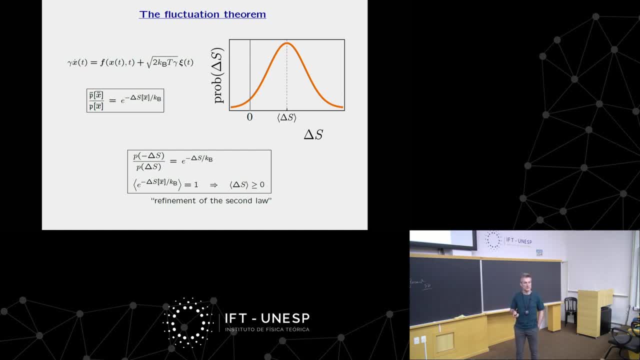 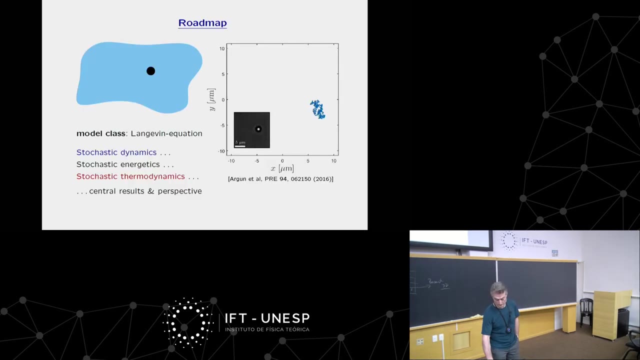 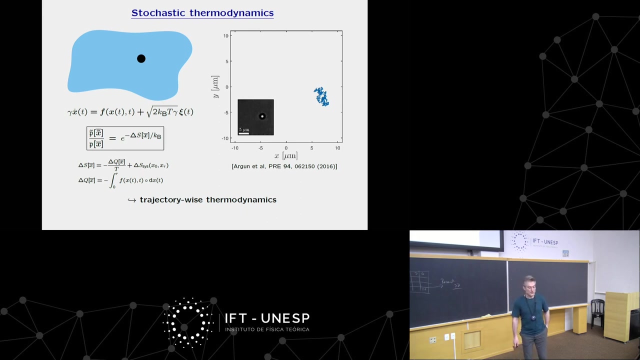 for observing this trajectory. in principle, When you use this parameter, noise, Gaussian noise, I don't remember. the parameter is why can I say the force moment is equal to zero? I don't got it, Because the Gaussian noise models the 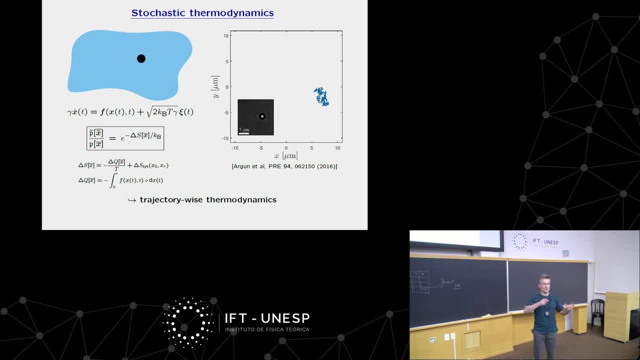 fluctuating effects of the thermal path, so the pushing around. And if the first moment of this noise were not equal to zero but had a finite value, then that would mean that the thermal fluctuations would push the particle in a specific direction, So it would move. 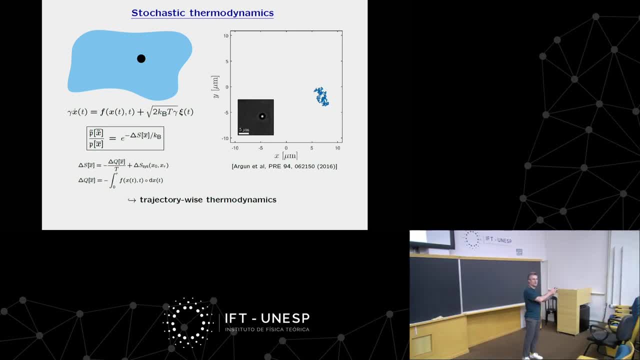 in a direction, just from the fluctuations in a certain direction, And this is not what you observe. The particle is not moving on average. Okay, So the first moment has to be zero. And how can I find this parameter statistically? How? 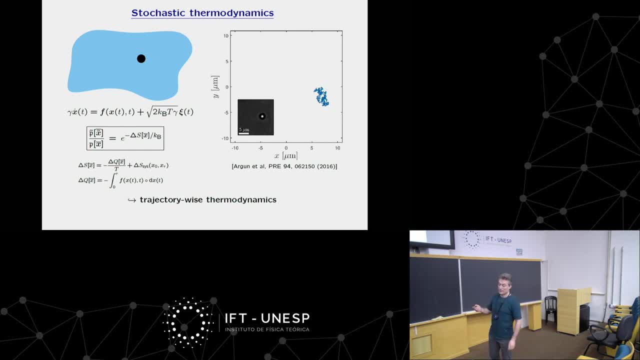 Where it comes from. Here's an example for the experiment. It's exactly like the action lab guy in principle, right? You see these things under microscope And then you take a movie of these trajectories and from that you get as data from the experiment. 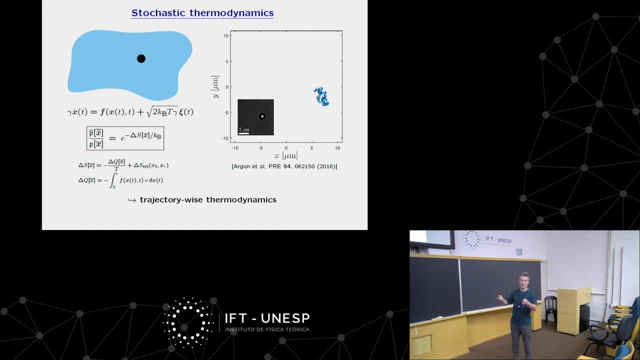 you get the position of the particle here in two dimensions, x and y, as a function of t. So you get all the trajectories And from that you can construct any distribution you like. Hello, Thank you for the lecture. Just a comment about: